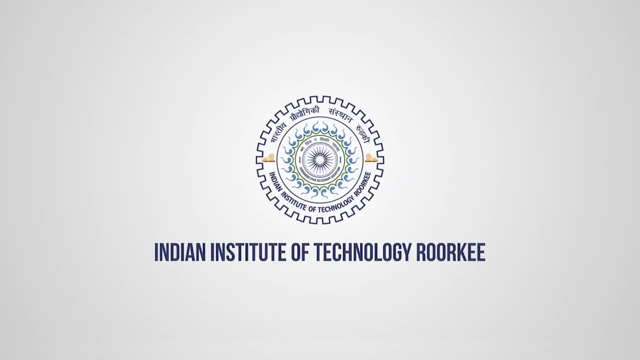 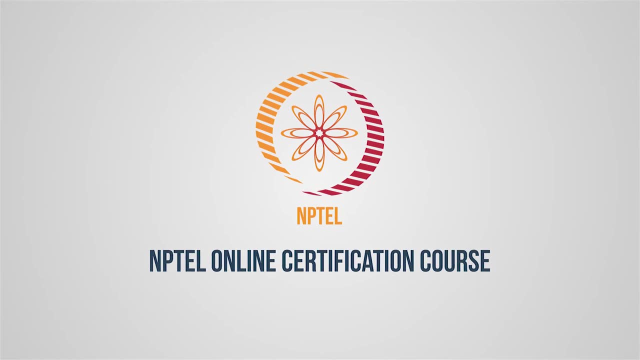 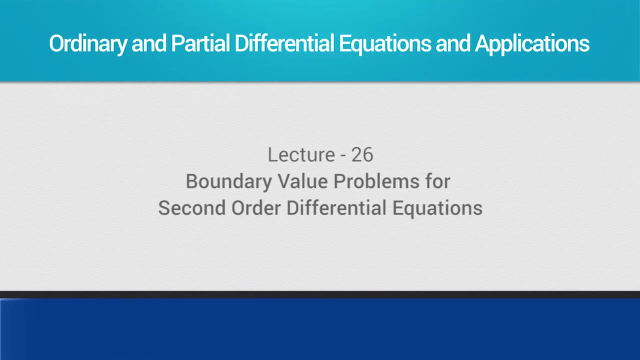 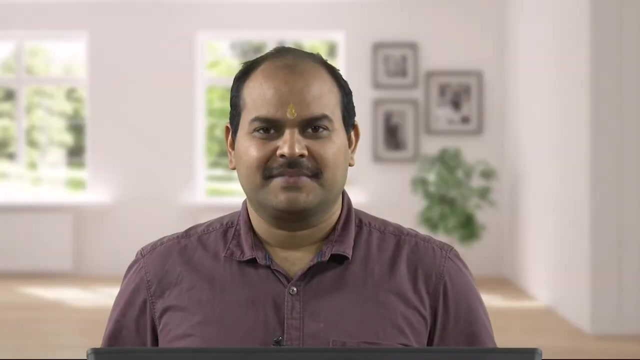 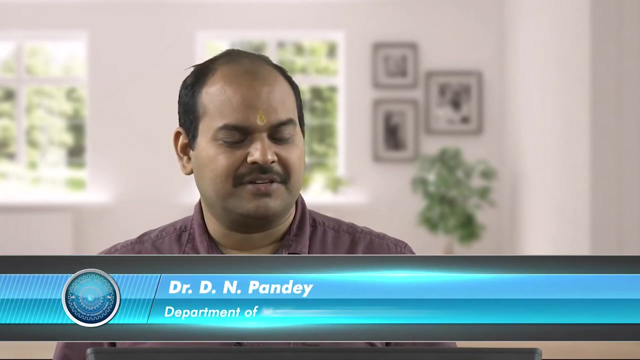 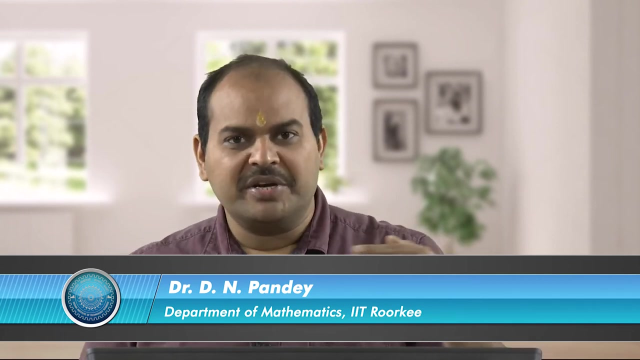 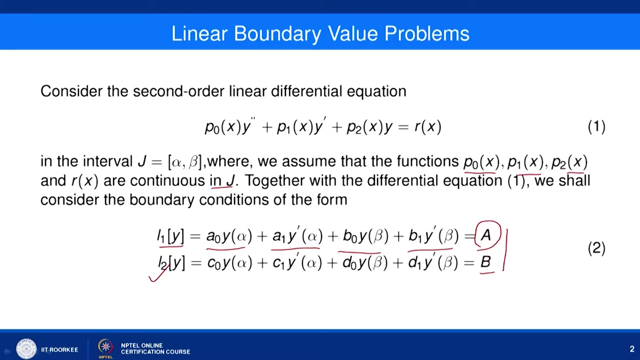 Hello friends, welcome to this lecture. In this lecture we will start our discussion of boundary value problems. So boundary value problems means equation is given and the conditions are defined on the boundary of the domain. So let us see what is the boundary value problem in a precise manner. So consider the second. 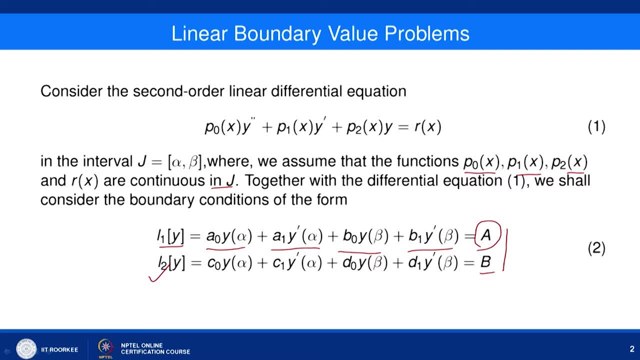 order: linear differential equation: p0 x, y, double dash plus p1 x, y dash plus p2 x y, equal to r of x here. So here coefficients p0, p1 and p2 are continuous in a interval j which is alpha to beta alpha. 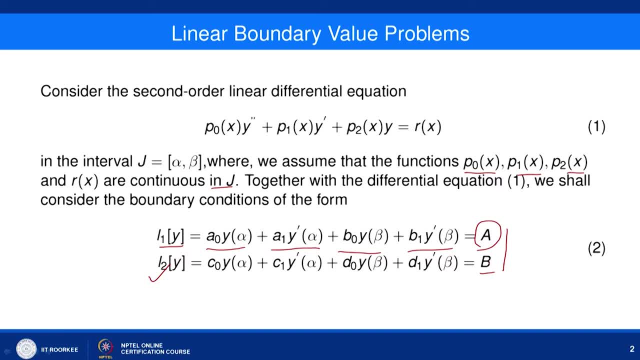 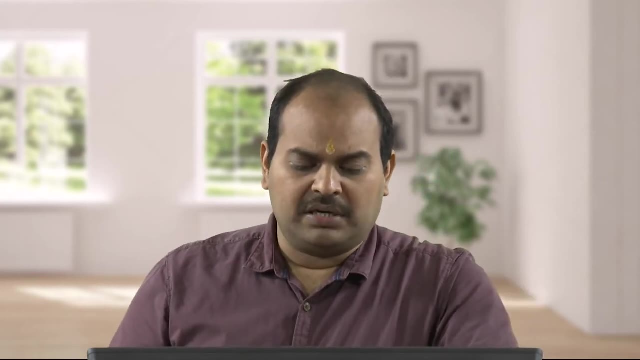 beta are any real numbers and alpha is beta. we will say Then we assume that function p0, p1 and p2 and rx are continuous in j. So by existence and uniqueness theorem we simply say that this solution exists If we are prescribed the initial condition along with this. But now let us consider the 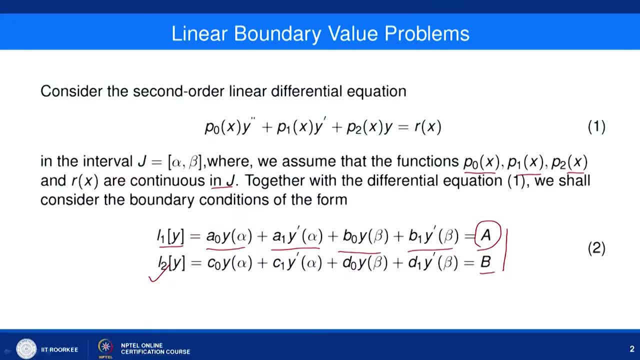 differential equation with the boundary condition like this: So here we define boundary condition of the form l1 y is given as a0 y alpha plus a1 y dash alpha, plus b0 y beta plus b1 y dash beta, and it is taken as some value, that is a. And second boundary condition is c0 y alpha. 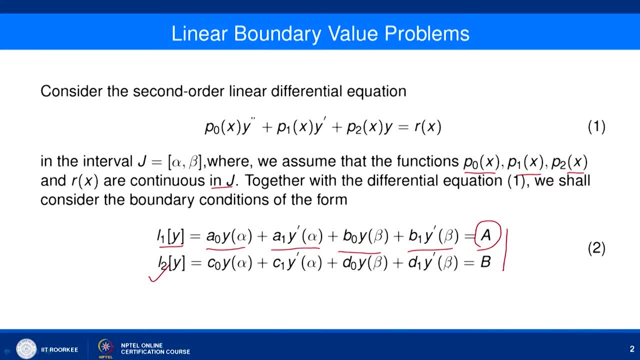 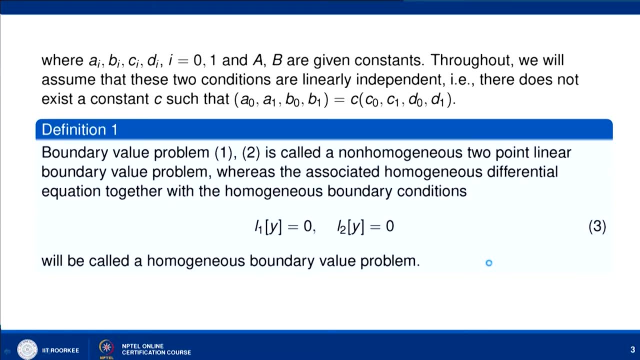 plus c1 y dash alpha plus d0 y beta plus d1 y dash beta x d2 y dash beta x d1.. Here a and beta c0-y plus c1 y beta. So here a i bi ci di, for i equal to 0 to 1 and a and. 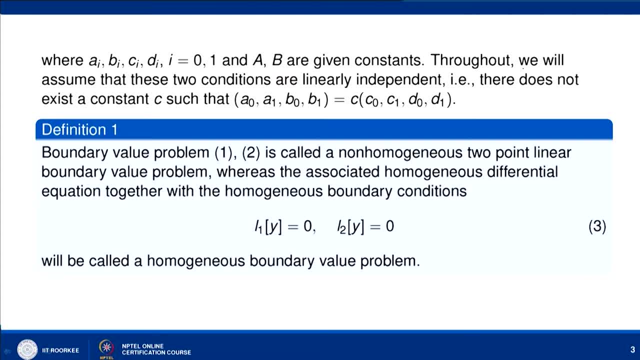 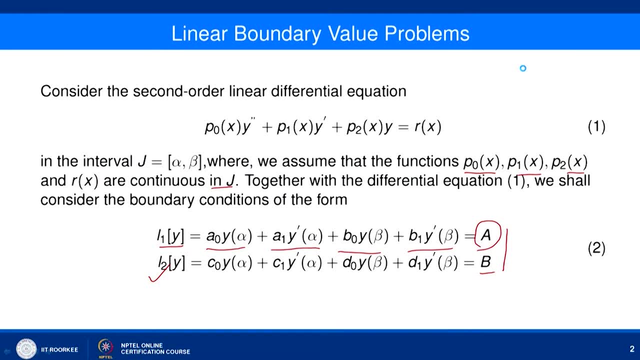 b are given constant, real constant, And throughout we assume that these two condition, the previous two conditions, are linearly independent. So we simply say that these are not precisely the same. So here we are, assuming that the vector a0, a1, b0, b1 are not scalar multiple of c0, c1, d0 and 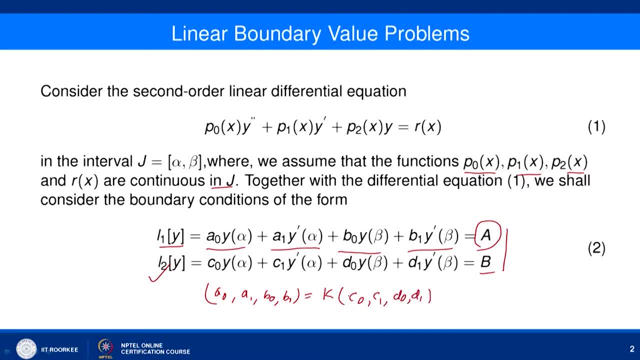 d1.. So it means that these 2 vectors are linearly independent vectors. So it means that we are precisely working with 2 boundary conditions rather than 1 boundary condition. So here I am assuming that they exist. no k, for which this is true. So it means that we are assuming that. 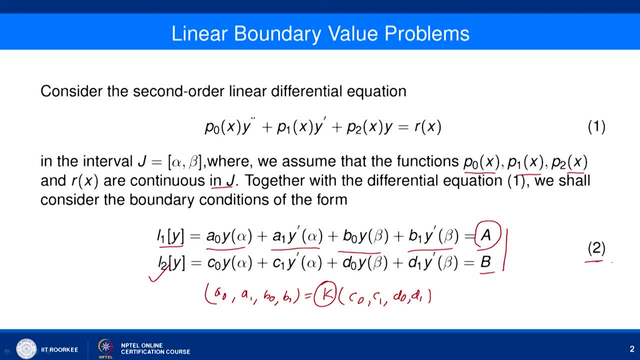 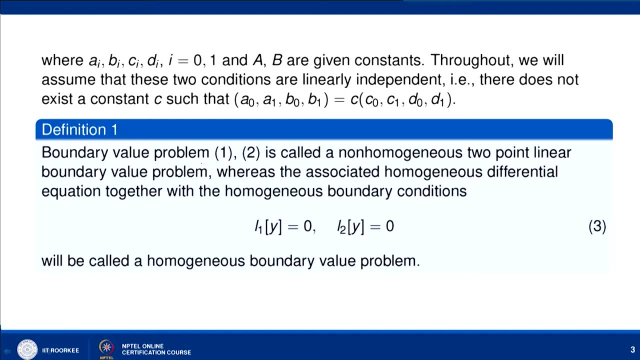 the condition given in 2 are linearly independent boundary conditions. So it means that now we define the boundary value problem. So boundary value problem 1, 2 is called a non-homogeneous 2-point linear boundary value problem, whereas the associated homogeneous differential equation. 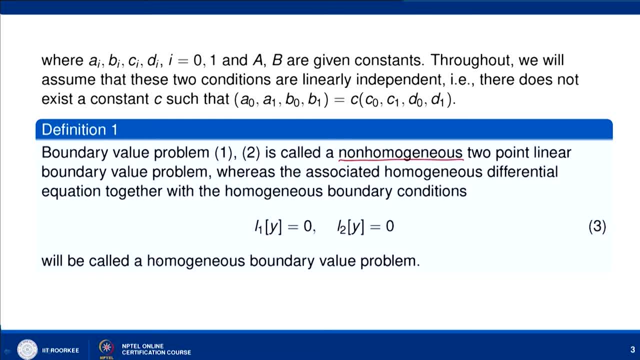 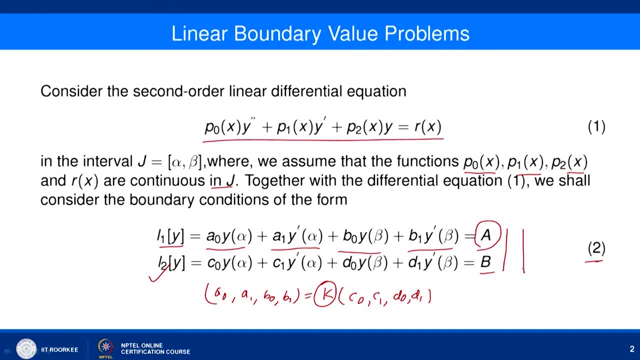 together with the homogeneous boundary condition, will be called a homogeneous boundary value problem. So first you just look at here: This is an equation and a boundary condition, because this condition is defined at 2-point: alpha one endpoint and beta is another endpoint. So we simply say that. 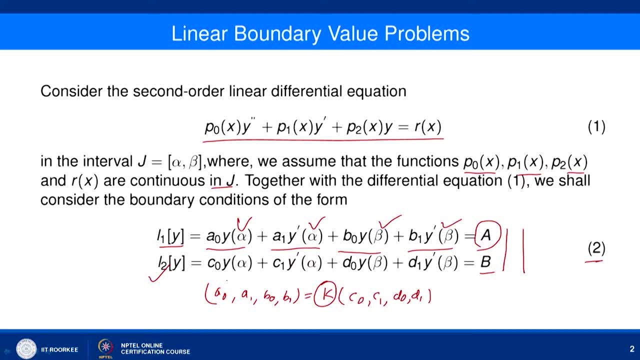 these L1y and L2y are conditions defined at 2 different point, that is, alpha and beta. So we say that L1y and L2y are boundary condition rather than initial condition, because it is defined at 2 different points. 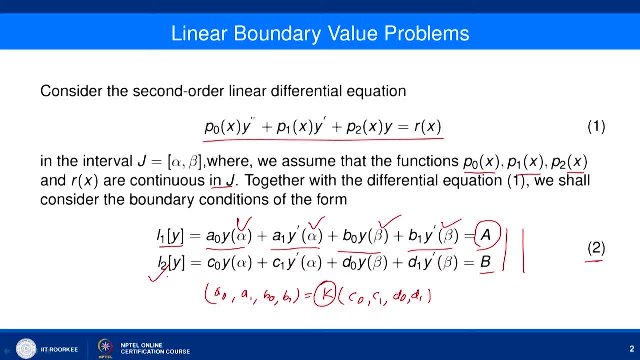 Say there are two different point. in fact, at the end point of this- So we call it boundary conditions or 2-point boundary conditions- It may happen that we have some more point on which we made defined condition in terms of more points. 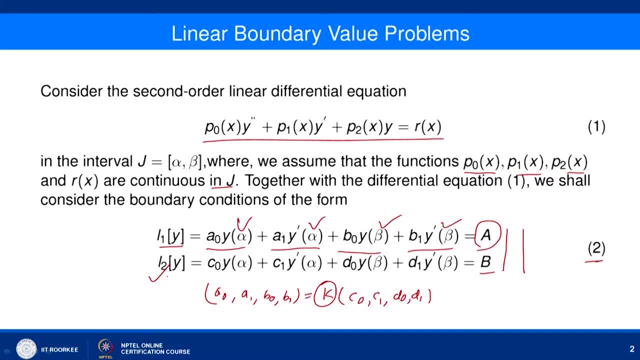 but right now it is a boundary or 2-point boundary value problem. Now we define non-homogeneous equation and non-homogeneous boundary condition. So if this Rx is non-homogeneous boundary condition, If rx is non-homogeneous, then we have 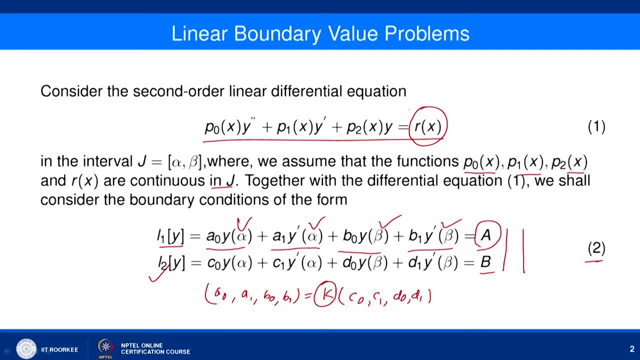 nth point: boundary are 0 in the whole interval, then we call it non-homogeneous differential equation. And if A and B are non-0 real constant, then we call these boundary conditions are non-homogeneous boundary conditions. So it means that if we consider non-homogeneous 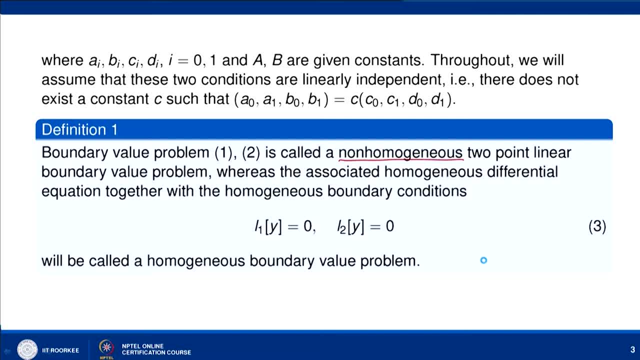 differential equation with non-homogeneous boundary condition. we call this as non-homogeneous two-point linear boundary value problem. But if we consider that Rx equal to 0 and A equal to 0, equal to B, we call it that this is a homogeneous boundary value problem. So it means that associated 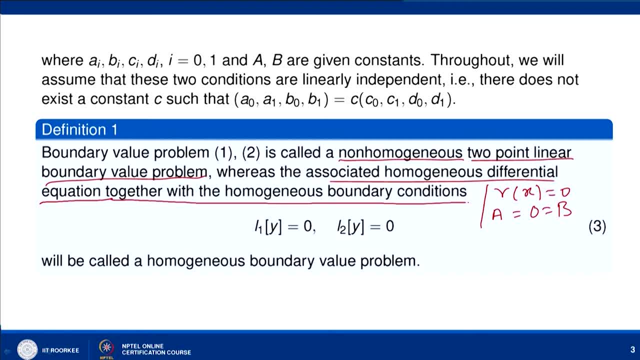 homogeneous differential equation, together with the homogeneous boundary condition, that is, L1y equal to 0 and L2y equal to 0, will be called a homogeneous boundary value problem. So it means that when Rx equal to 0.. A equal to 0, A equal to B, then in this case we call this as homogeneous boundary value. 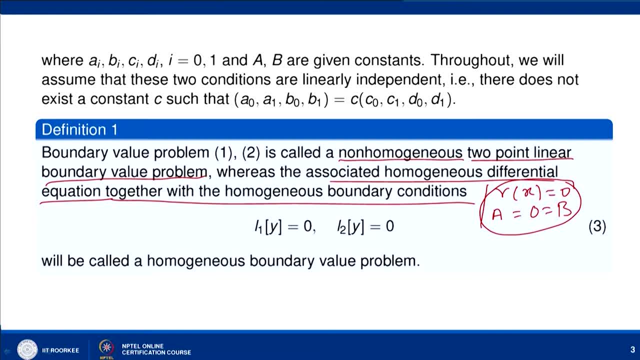 problem. But if Rx is non-0, A and B are non-0, then we call it non-homogeneous boundary value problem. okay, In fact, one of A and B has to be non-0 in non-homogeneous boundary value problem. 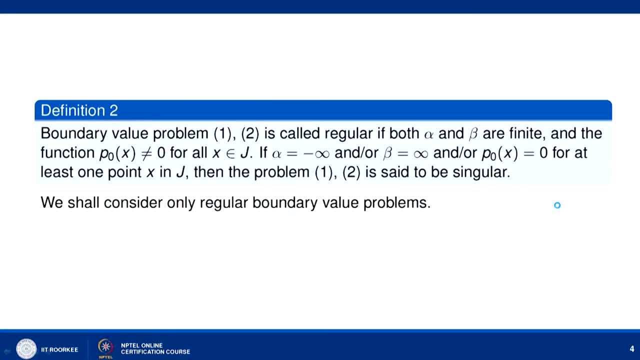 Now we define regular boundary value problem and singular boundary value problem. So we simply say that boundary value problems 1 and 2 is called regular if both alpha and beta are finite and the coefficient P0x- coefficient of d2y by dx, square this P0x, this is non-0 in the entire interval j. So if interval is: 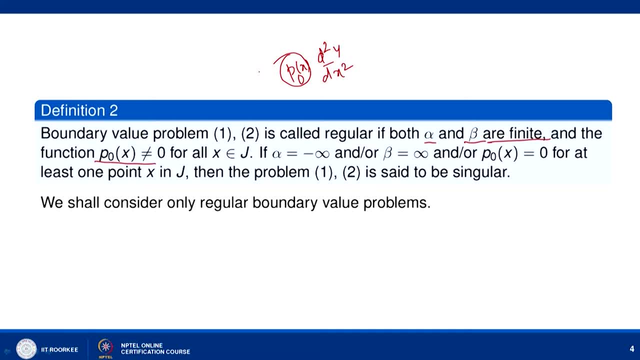 finite and the coefficients are non-0, then we call our boundary value problem as regular boundary value problem. Otherwise we call our boundary value problem as non-homogeneous boundary value problem. It means that if your alpha is minus infinity and or beta, and or or beta equal to infinity. 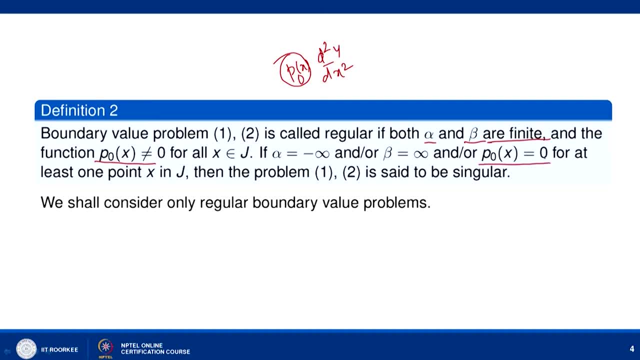 and or or P0x equal to 0 for at least one point in j, then the problem 1 and 2 is said to be a singular boundary value problem And for this particular course we will consider only the regular boundary value problem. It means that we consider that our endpoints 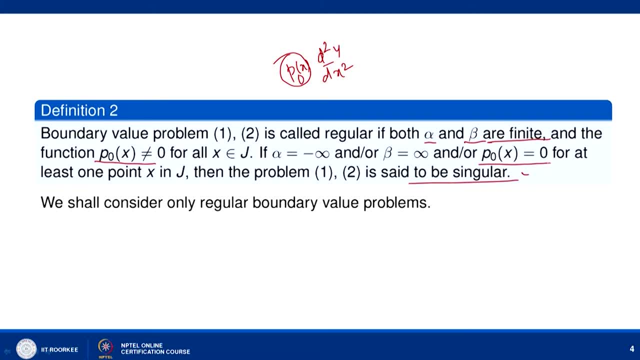 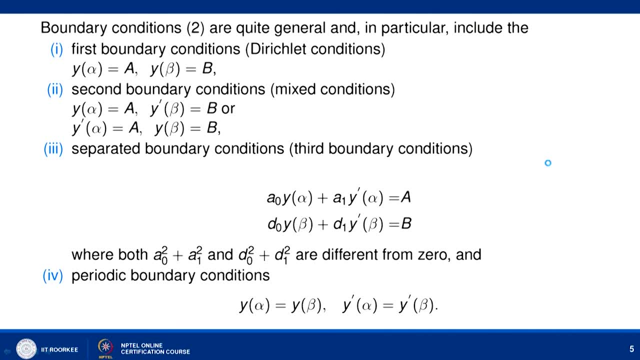 are finite and the coefficient of d2y by dx square is non-homogeneous. and the coefficient of d2y by dx square is never 0 in the set interval: infinite, finite interval. Now, the boundary condition which we have considered: L1y equal to a and L2y equal to b are very 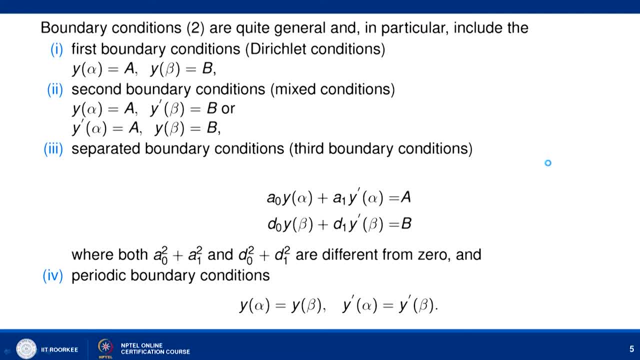 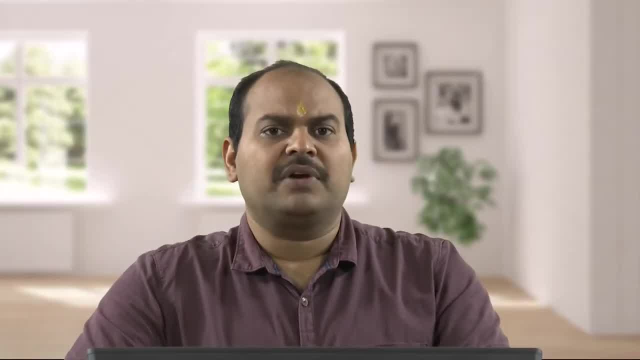 general boundary conditions and we can summarize and we can write many more boundary condition as a special case of L1y and L2y. So first let us see what is the boundary condition of L1y and L2y. So first let us 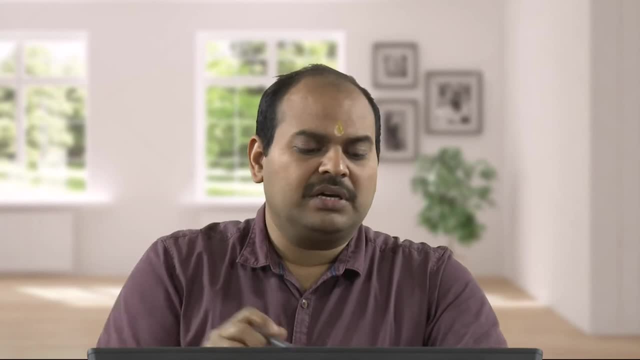 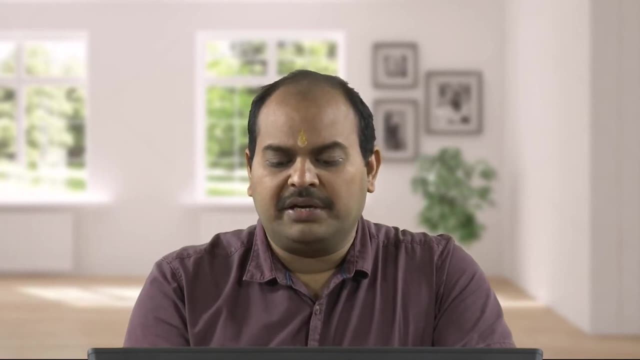 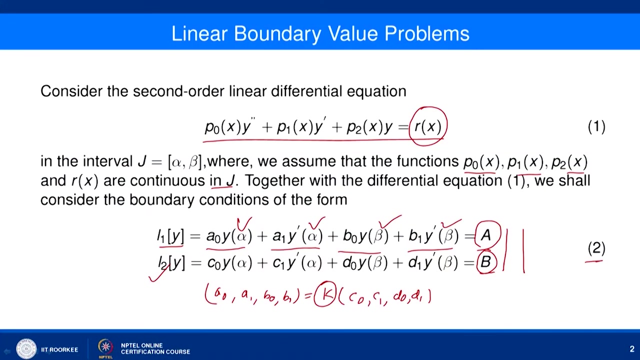 take a special case where L1y is given as y alpha equal to a. So here L1y is y only. So here L1y, which I am writing, as here we are simply taking L1y, is basically taking only a0 as 1, rest all 0. So we say that the simplest form of L1y is that a0 is equal to. 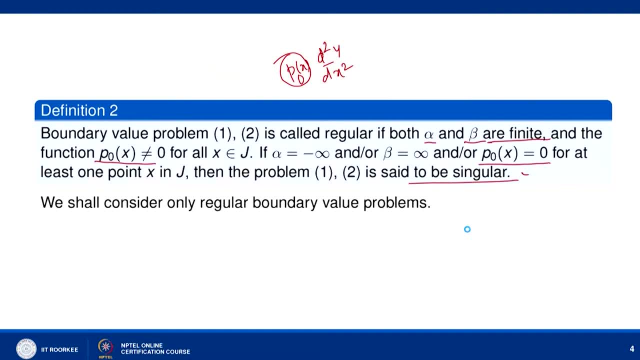 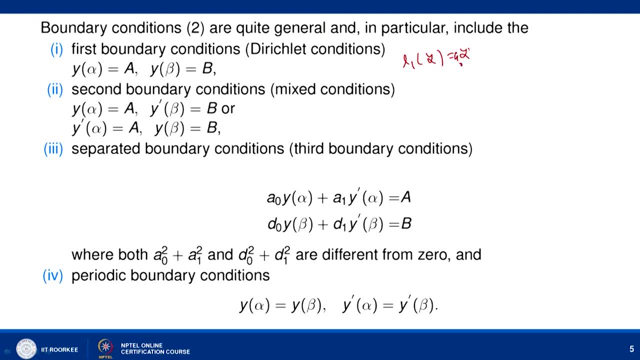 1, rest all simply 0. So here L1y is equal to simply y only. So here we simply say a0 is equal to 1.. So y alpha and all are 0.. 0 y dash alpha plus 0 y beta, plus 0 y dash beta. So it is a particular. 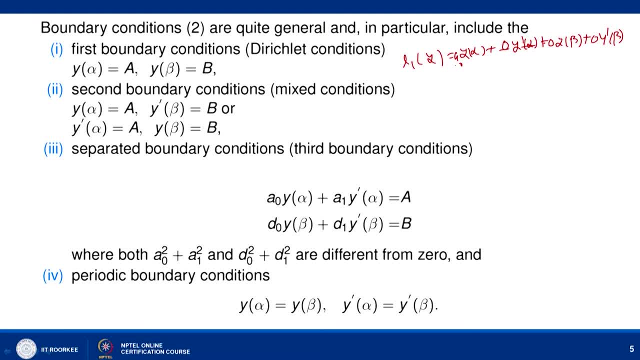 case of your L1y. So here we simply assume that a0 equal to 1, rest all 0. Similarly, you assume that c0 is equal to 1, rest all 0. So we have boundary condition: y alpha equal to a and y beta equal to b. So we say that: 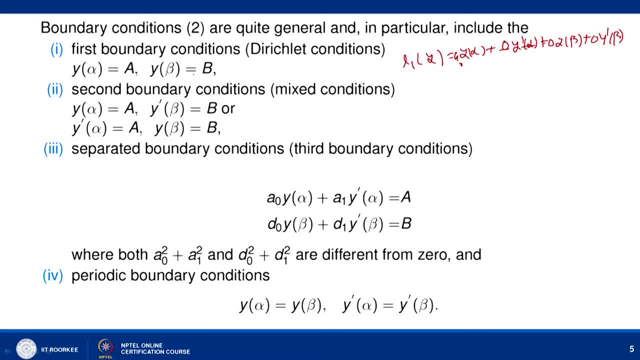 it is first boundary condition, and sometimes we call it a Desolate condition. So here, in first boundary condition or Desolate condition, your function is given some value at the end point. And then second boundary condition, which we call as mixed boundary conditions, where function as well as its derivative, is defined at the end points. So here one kind. 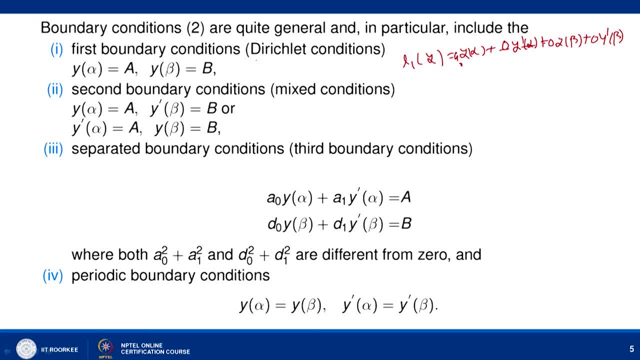 of mixed boundary condition is: y alpha is given as a and y dash beta is equal to b. So it means at one point your function is given and the other point your derivative is given. So y alpha equal to a, y dash beta equal to b or the other way, that is y dash. 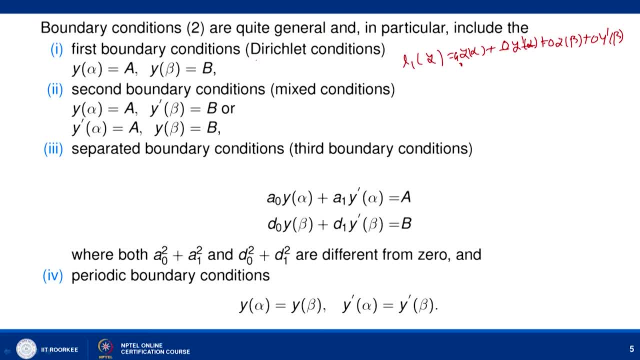 alpha equal to a means. at the end of x equal to alpha, your denominator is given as beta, truthfulative derivative is given a particular value and the other end, the function is defined or getting a particular value. So this is your second boundary condition, or we say mixed condition. 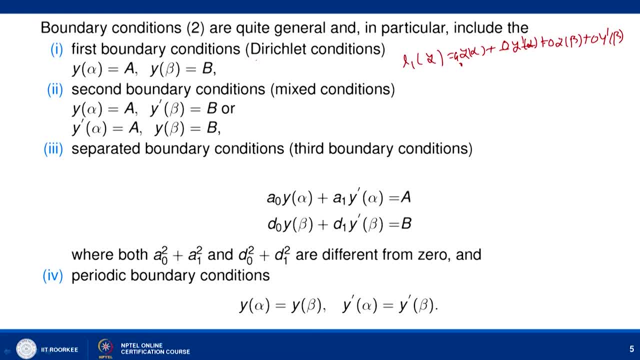 Now third, that is separated boundary condition. so it means that here one condition is given in entirely at one point, one end point, and other boundary condition is given at the other end point. So here your L1y is defined only at say alpha, x equal to alpha. So we say a0 y alpha plus a1 y dash. 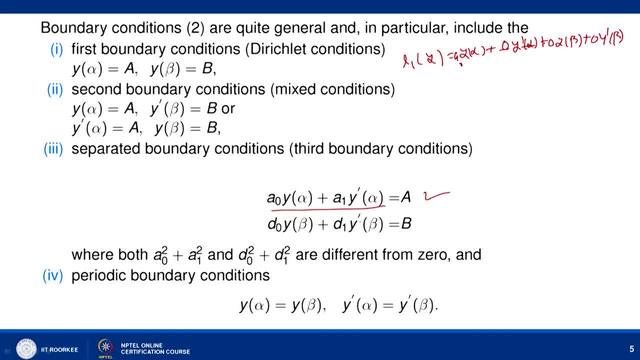 alpha, equal to a and d0 y beta plus d1 y dash beta, equal to b. So here a0, a1 is some nonzero and b0 and b1 are 0.. Similarly, in L2y your c0 and c1 is given as 0 and d1 and d0 is 0. 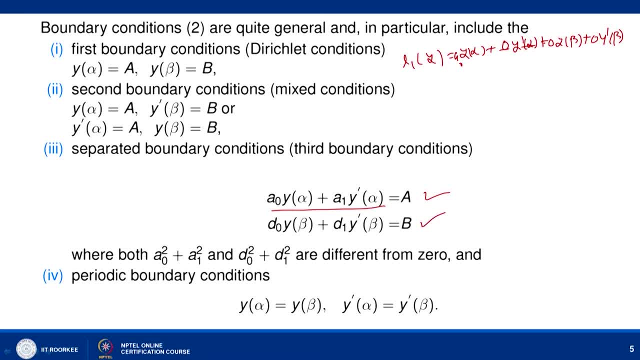 and d1 are nonzero values. So here we say that your first boundary condition is defined only at x, equal to alpha, and the second boundary condition is defined only at the other point, that is, x equal to beta. So your boundary conditions are separated, So we call these: 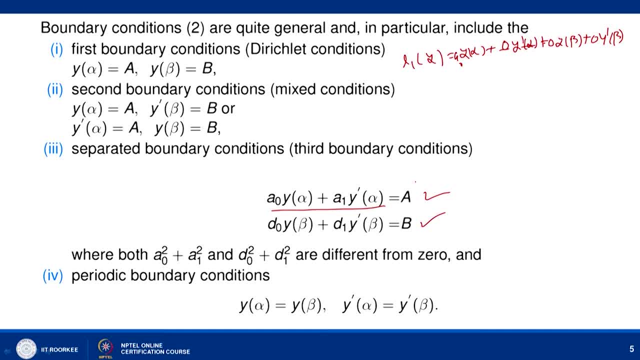 boundary conditions are separated boundary conditions, and here we are assuming that not all a0, a1 is 0. So we assume that a0 square plus a1 square is different from 0, and similarly d0 square plus d1 square is different from 0. here Then there is one more very important kind of 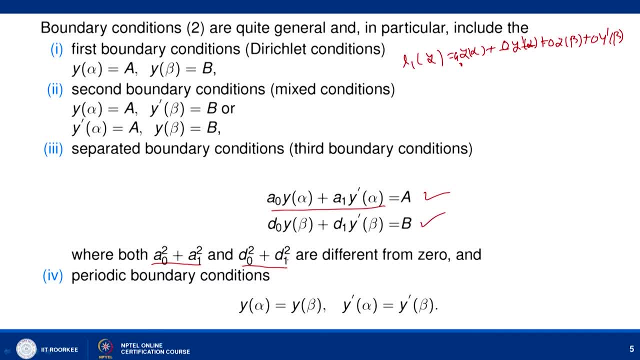 boundary conditions, that is, periodic boundary condition. So it means that the initial point is the same as final point. So it means that the value of y given at alpha is same as given at beta, So y alpha is equal to y beta, and similarly the derivative, So the value of derivative at 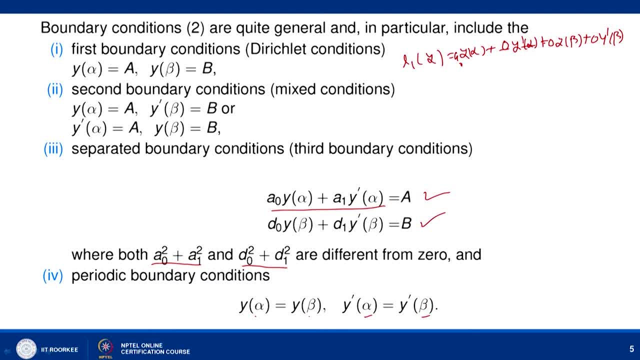 alpha is same as the value given at the final point. So here y alpha is equal to y beta and y dash alpha is equal to y dash beta is. these kind of conditions are known as periodic boundary condition. So the initial point, the value given. 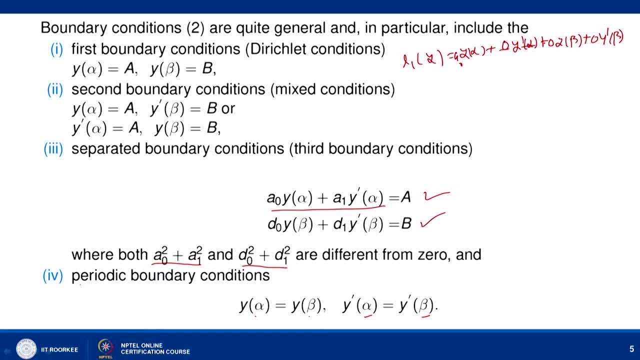 at initial point is same as the value given at the final point. So it means that y alpha is equal to y beta and y dash alpha is equal to y dash beta. So these are some important boundary conditions which we need to discuss very often. Now let us consider the boundary conditions. So let us 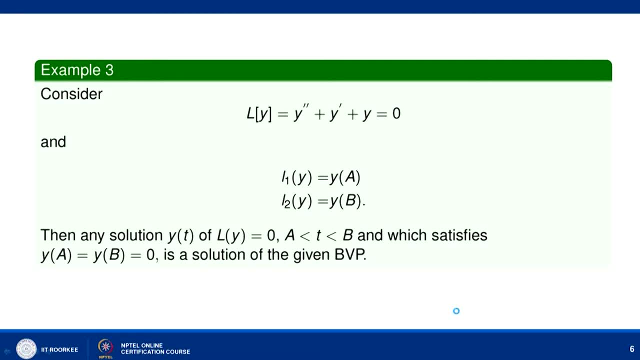 consider one example. So let us take a differential equation. say y double dash plus y, dash plus y equal to 0, and here boundary conditions are separated boundary condition- and it is a drizzled kind of boundary condition that is y equal to y of a and l to y is equal to y of b. 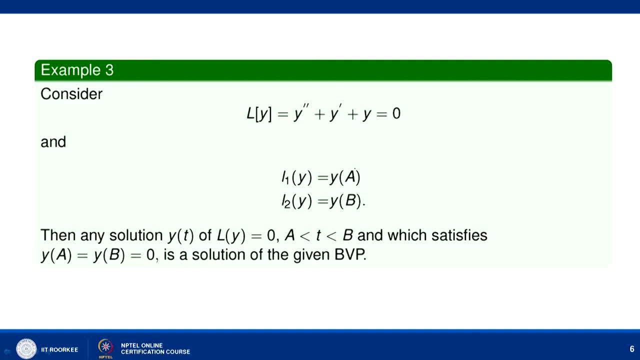 So it is the first kind of boundary condition and it is also a separated boundary condition, and so we can write the solution of this which satisfy. the conditions at a and b are simply a solution of this. So, in particular, if I take your y a equal to 0 and y b equal to 0, we can say that solution. 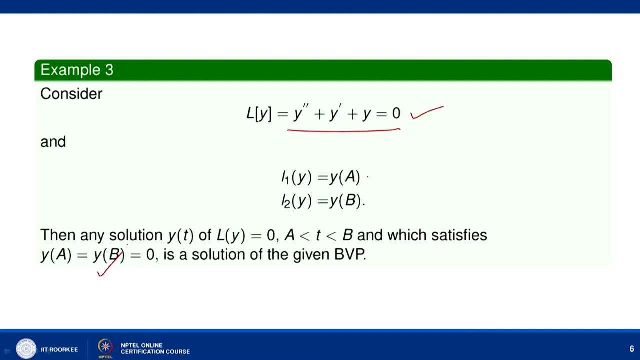 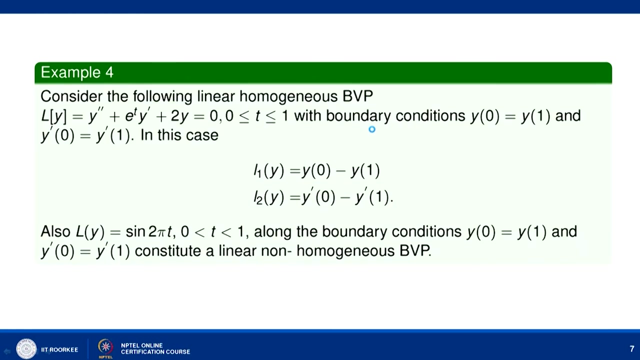 of this. satisfying this is a solution of the given y b, So we simply write it: 0.. So it means that any solution which satisfy this and these conditions are known as the solution of this boundary condition, And in fact this is a homogeneous boundary value problem. Then consider the next example. Here we 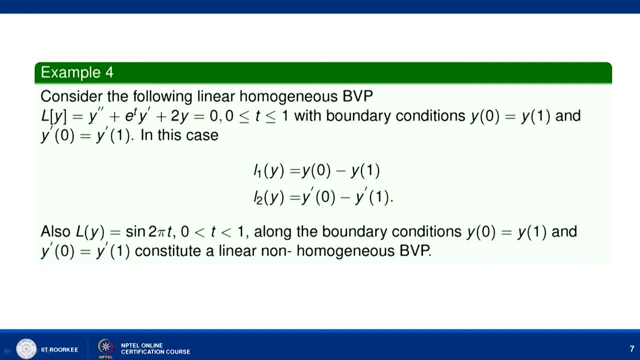 have a homogeneous boundary value problem. So y double dash plus et, y dash plus 2y equal to 0 and t is lying between 0 to 1.. Boundary conditions are this: y0 equal to y1 and y dash 0 equal to. 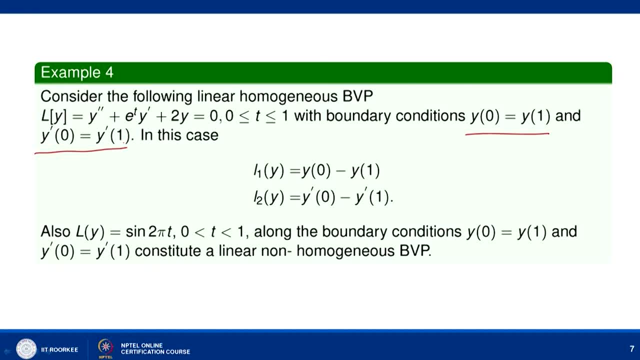 y dash 1.. If you recall, this is a periodic boundary conditions And here let us write this: y0- y1. this as L1y equal to y0 minus y1, L2y as y dash 0 minus y dash 1.. 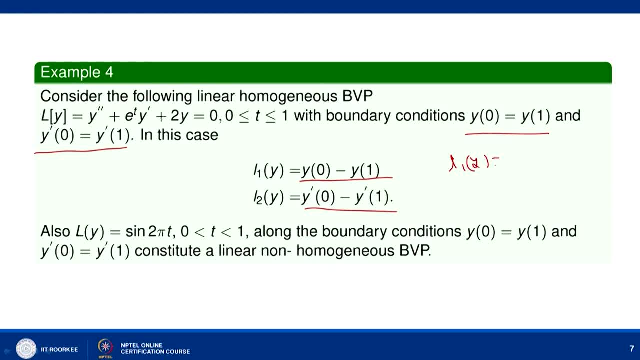 So here L1y equal to 0 and L2y equal to 0, give you these periodic boundary condition which is defined like y0 equal to y1 and y dash 0 equal to y dash 1.. So we can simply say that if you take any 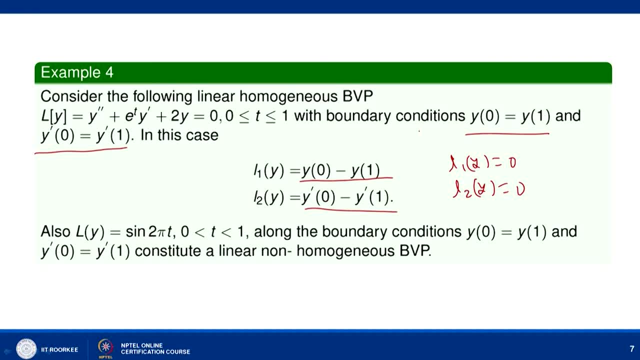 say non-homogeneous boundary value problem. So if you take any non-homogeneous boundary value, that is ly equal to sin 2 pi t. or you can say y double dash plus ety dash plus 2y, equal to sin 2 pi t, along with the boundary condition that is y0 equal to y1 and y dash 0 equal to y dash 1.. 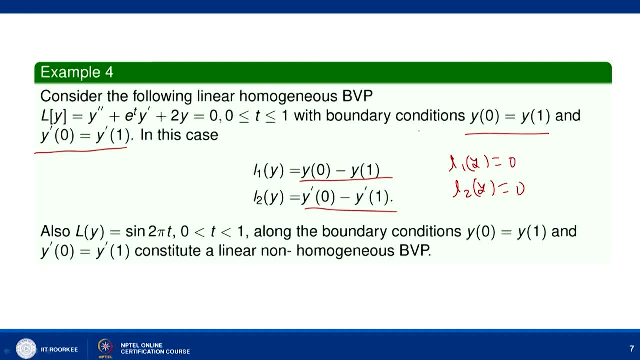 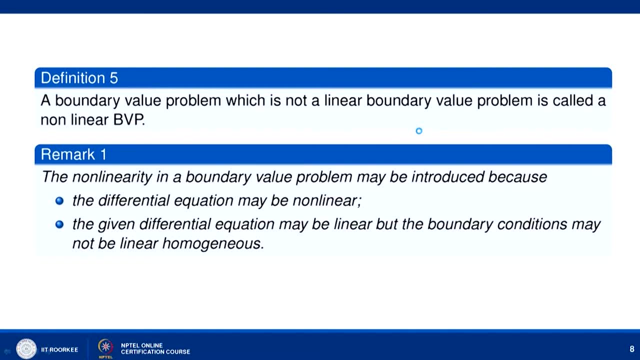 This will constitute a linear, non-homogeneous boundary value problem. So these are example of some boundary value problem and some boundary conditions. Now we again define the classification of boundary value problem in terms of linear, non-linear. so a boundary value problem which is not a linear boundary value problem is called. 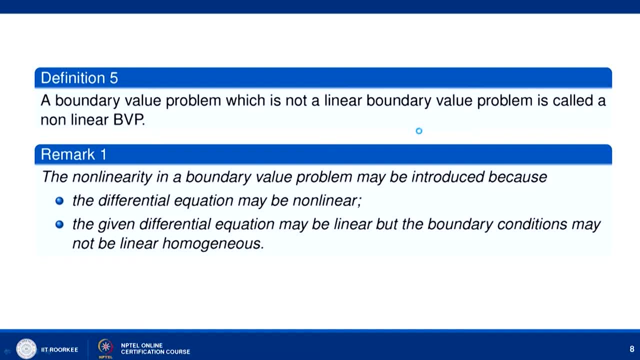 a nonlinear boundary value problem. and this is happening because this nonlinearity in a boundary value problem may be introduced because of the following thing: the first thing is the differential equation may be nonlinear. So here we have 2 components. one is differential equation. 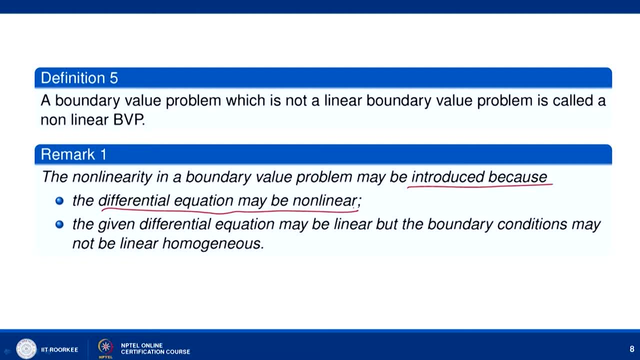 and the other is a non-linear system. So, for example, we have differential equation individuals where there are only two elements: i is that is the differential equation which is non-linear, and other component is your boundary conditions. So your nonlinearity, boundary value problem. 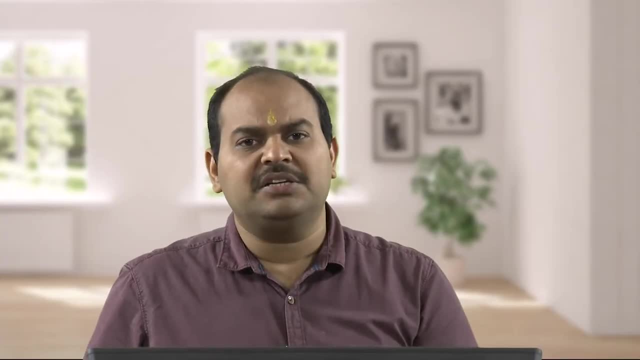 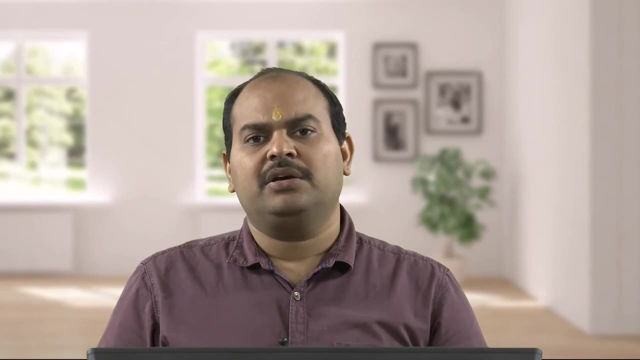 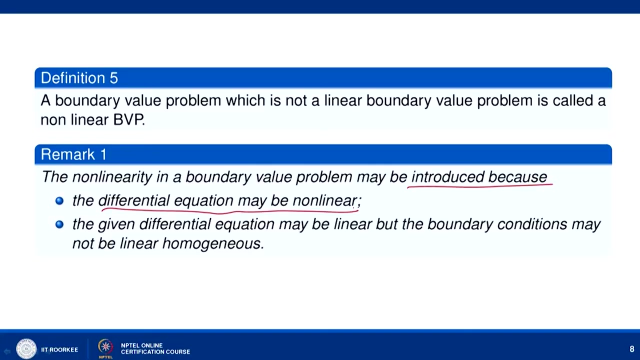 is said to be linear if both the equation as well as the conditions are linear, and if any of these two fail, then we call this as a nonlinear boundary value problem. So it may happen due to that, differential equation may be nonlinear and the given differential equation may be linear, but the boundary condition may not be linear. So we 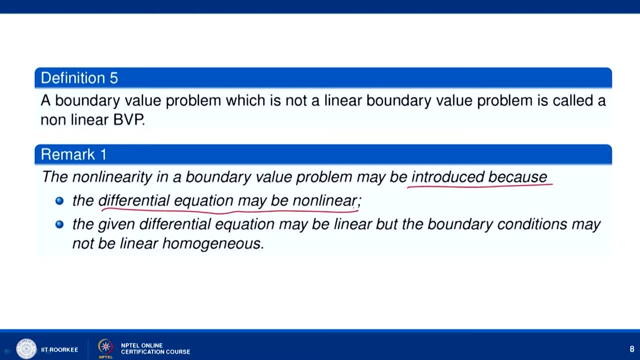 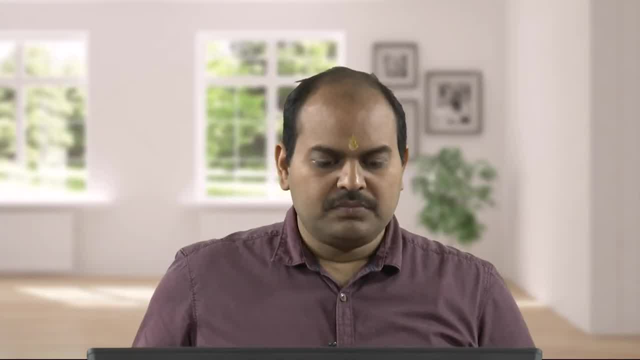 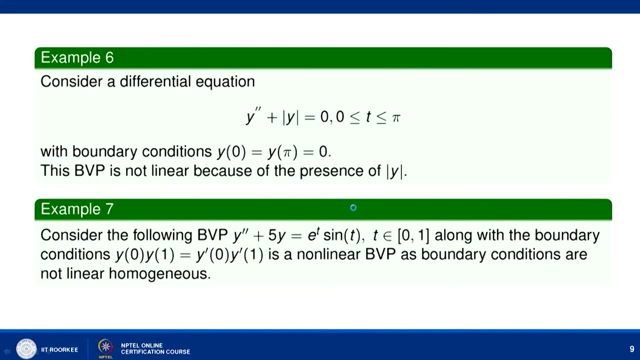 simply say that nonlinear boundary value problem is maybe because of equation may be nonlinear or the condition may be nonlinear. So let us consider some example of nonlinear boundary value problem. First problem is y double dash plus mod of phi equal to 0. here t is defined from 0 to phi here and boundary condition is: 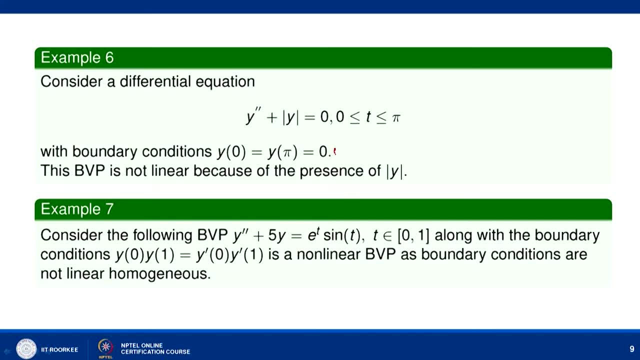 0 equal to y, pi equal to 0.. So these are conditions which are defined on the boundaries and if you look at these, are very simple boundary conditions, separated boundary conditions. but if you look at the equation, equation contain your modulus y terms, so it is a nonlinear differential equation. 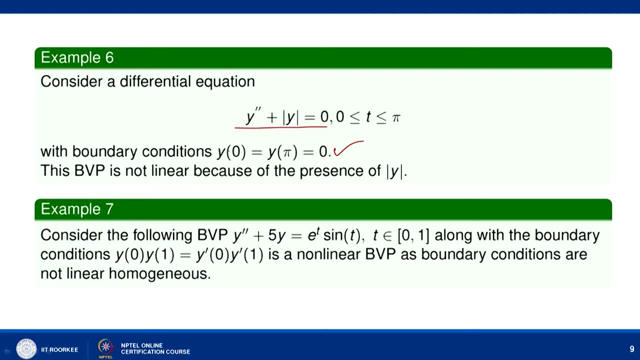 Your boundary conditions are linear, but equation is nonlinear. So we simply say that it is a nonlinear boundary value problem, and I hope that you already know how to check whether it is a linear, nonlinear boundary value problem. For that you define operator Ly as this: y, double dash plus. 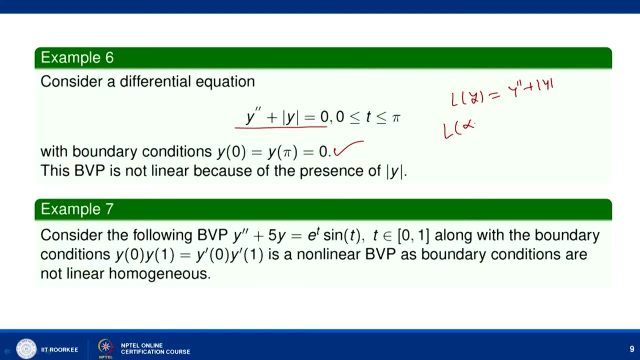 mod of y and you check that, if L of alpha y1 plus beta y2, if it is equal to alpha L of y1 plus beta L of y2.. If these holds, then we call it linear, and if this does not hold, we call it nonlinear. and if you check, 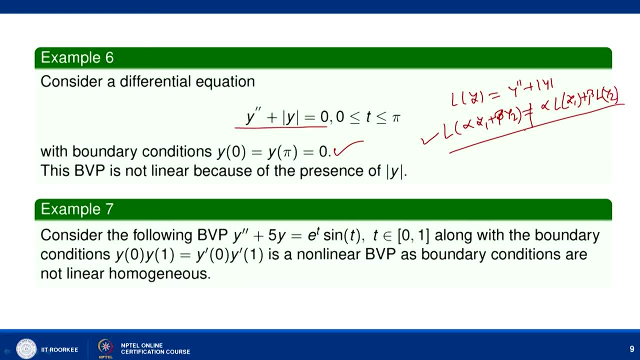 that here it is not holding. So you can check that differential equation is not a linear differential equation. So we call this problem as nonlinear boundary value problem. Now look at the next example. here boundary value problem is y, double dash plus yy, equal to e, to power t, sin t t is 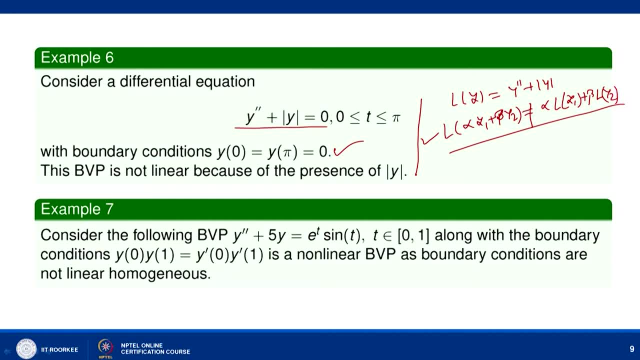 again in some interval. Let us see say 0 to 1, along with the boundary condition y0 into y1 equal to y dash 0, equal to y dash 1.. So here, if you look at, your boundary conditions are not linear. So we simply say that your 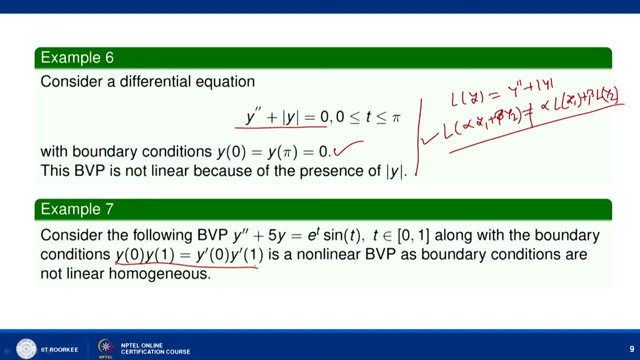 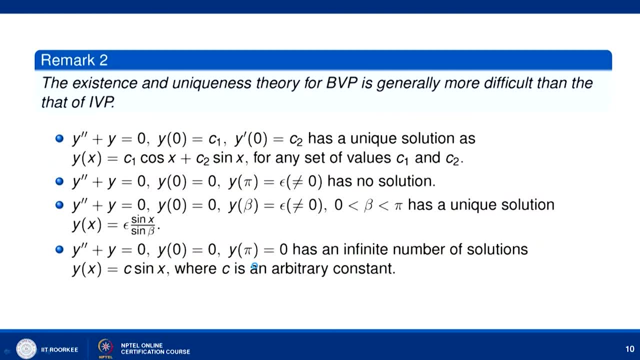 equation is linear, differential equation is linear, but boundary condition is not linear, So we again call this as a nonlinear boundary value problem. Now why again we are discussing the boundary value problem different from initial value problem? because we have already discussed the initial value problem. we have discussed the existing uniqueness theorem and 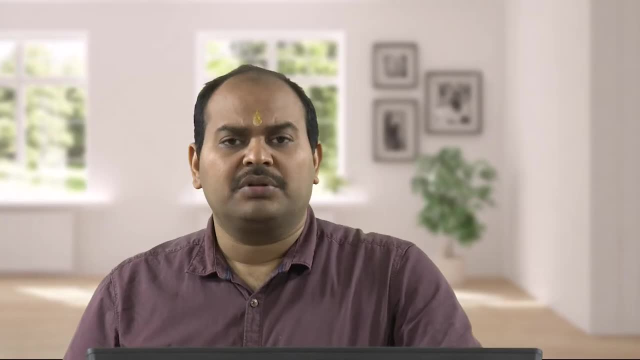 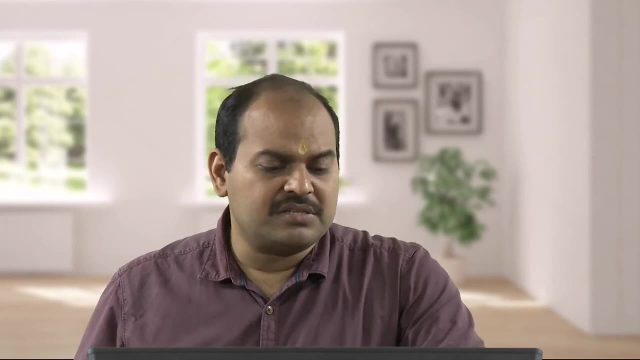 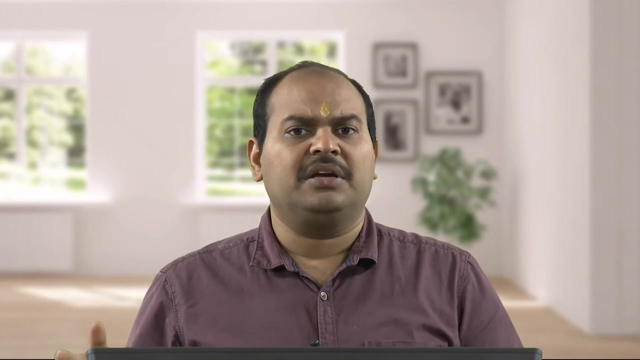 consider several method to find out the solution of initial value problem, but why we are bothering about boundary value problem? So we can say that the existence and uniqueness results of boundary value problem is, in general, quite difficult than the theory of initial value problem, For example. 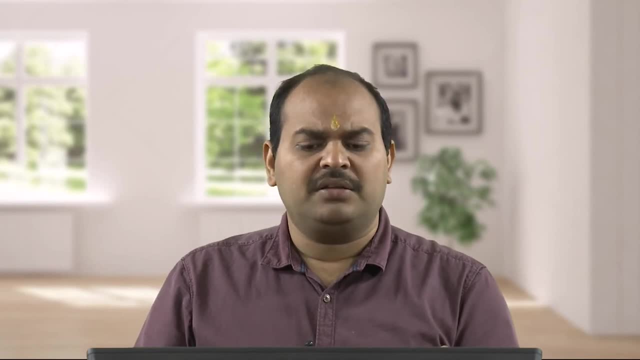 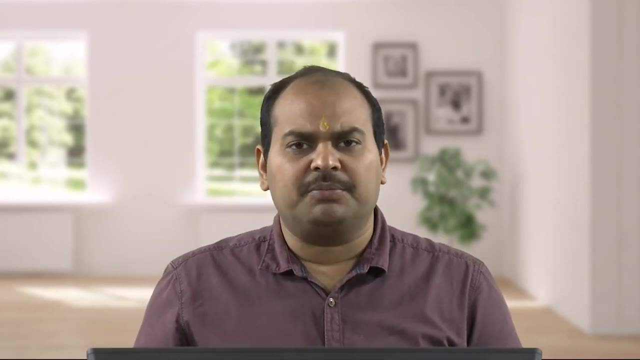 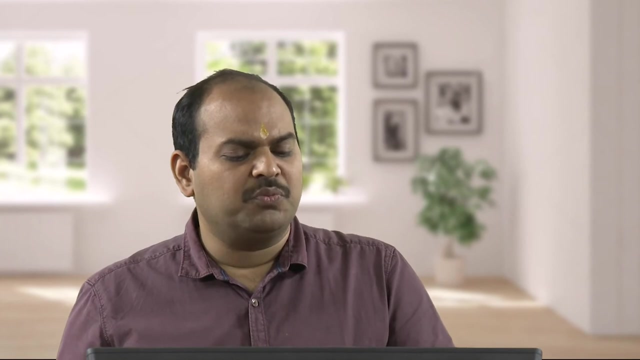 take very simple example and try to understand why this theory of existence and uniqueness for boundary value problem is, say, difficult than the initial value problem. So first let us take simple example: y double dash plus y equal to 0. and take the initial condition: y0 equal to c1 and y dash. 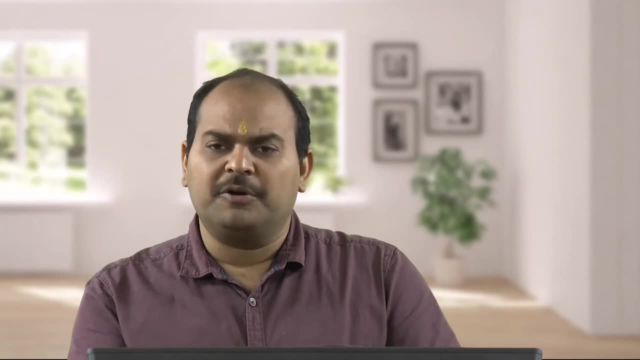 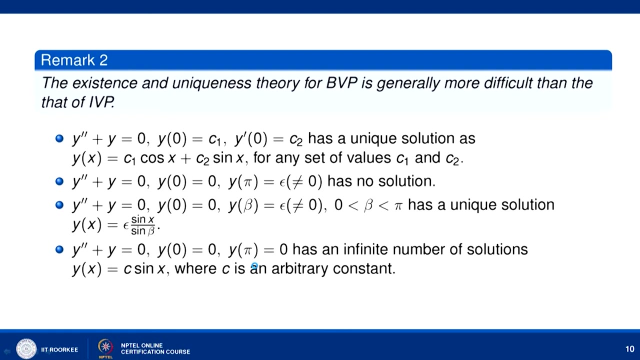 0 equal to c2.. This is a simple initial value problem and we know the solution is given as yx equal to c1, cos of x plus c2, sin of x, and you can take c1c2 and you can get your solution in very nice way and the solution is also given. 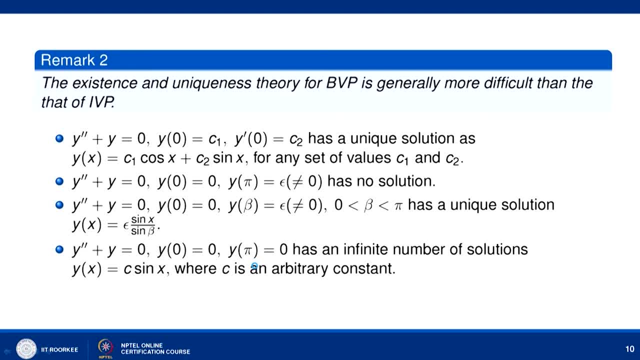 But now let us, in place of initial condition, now let us define boundary condition and see that how this nice solution is change into difficult solution. So equation remains the same, that is, y double dash plus y equal to 0. but now your boundary conditions are changed. 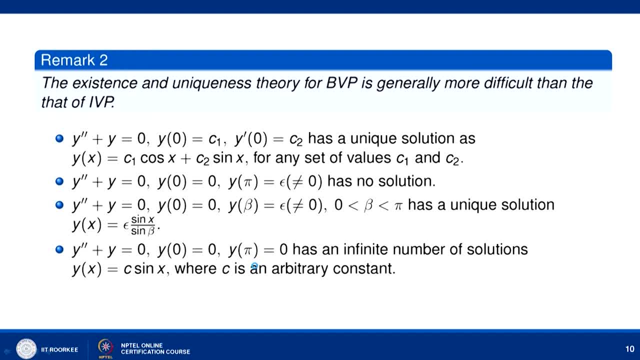 Your boundary conditions are y0 equal to 0 and y phi equal to some epsilon, So some value. epsilon may not be so important because extremely different sacar not be 0 value and we can see that it has no solution at all. How we can check that it has? 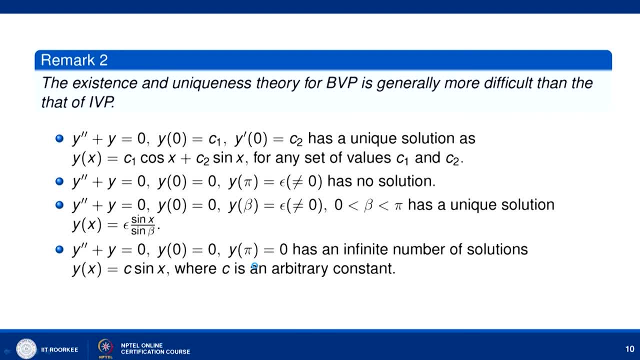 no solution. So what we try to do? We try to solve this equation for a general initial condition. So we simply say that your yx is equal to general solution of this differential equation is c1 cos of x plus c2 sin of x. and we want to find out this c1 and c2, but not with the help of initial. 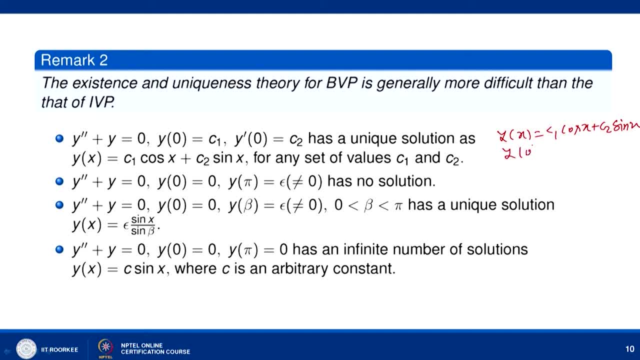 condition, but with the help of boundary condition. Now we look at y0 equal to 0. This force has to choose c1 equal to 0, right, because if you put x equal to 0, then sin x is 0 and cos x is 1,. 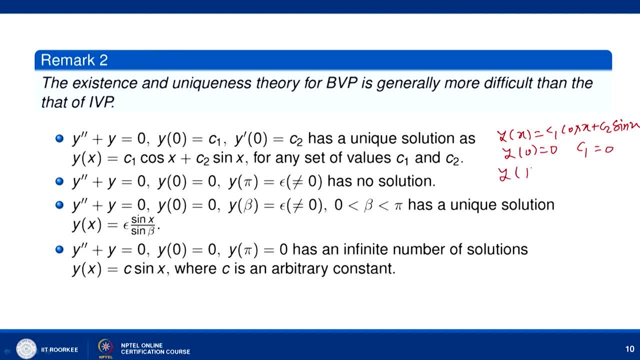 so c1 has to be 0, and. but if we look at ypi equal to epsilon, then look at here What do you have? This is epsilon equal to c1 and c1 is 0. So it is c2 sin of pi. Now, sin of pi is simply 0, but here we have a nonzero value, So it means 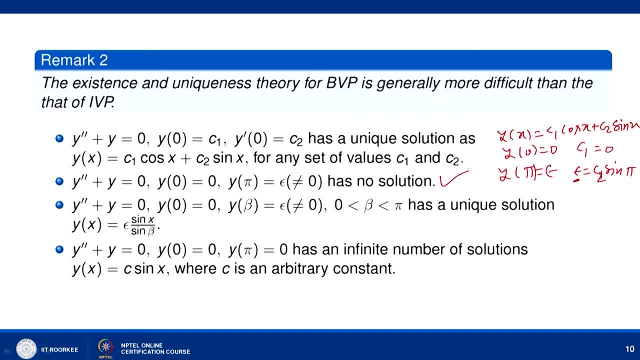 that this has no solution, right? So simply say that when y of pi is some nonzero value, then it has no solution, right? But suppose you look at this case that here y double dash plus y equal to 0, y is equal to 0, ypi equal to 0. Now here we have taken the value epsilon. 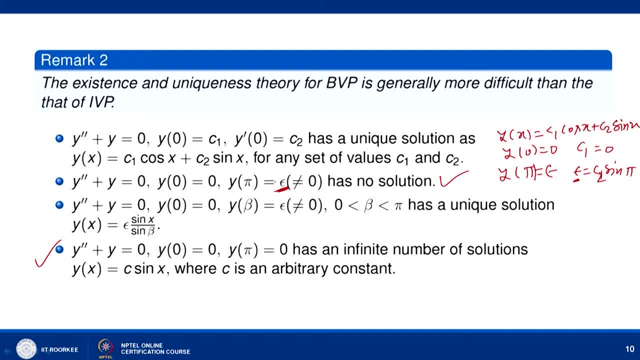 But if you take epsilon, maybe any value, maybe very, very small, but still it will have no solution. but if you take epsilon as 0, then we can easily check that it has an infinimany solution. That is quite say very say strange thing, because here we just differ our boundary condition by 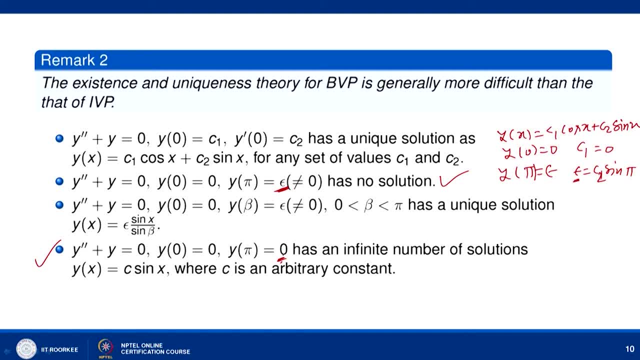 a little. So this epsilon may be very small quantity, but still in one case we have no solution. but in other case we have infinimany solution and you can easily find out the infinite many solution, as here, if you look at in place of 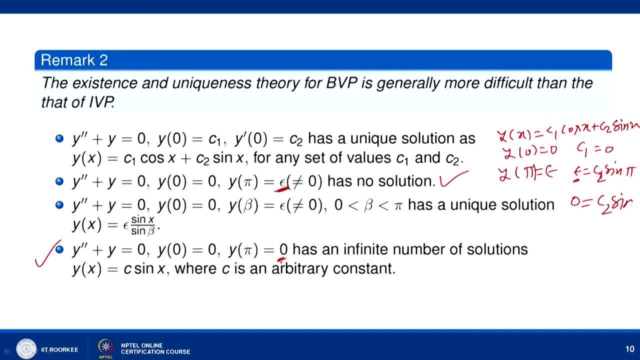 epsilon, if you put 0, then 0 equal to c2 sin pi. of course this is 0, so I can take any value of c2, right? So it means that we have infinite many choices for this c2 and we can say that our 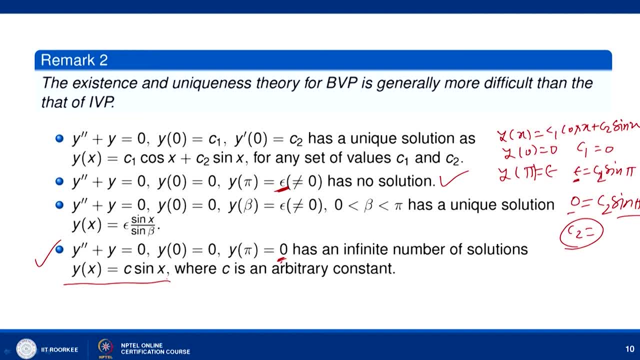 solution is given as yx equal to c sin x and you can take any value of c and you take different value. we have a different solution of this. So here we say that we have just changed the boundary condition a little, but we have in place of no solution. now we have infinite many solutions. 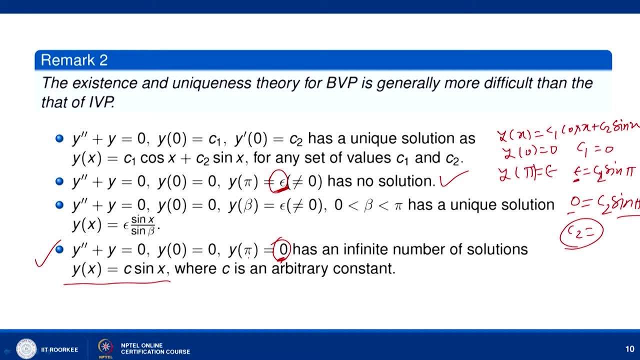 So that is very strange for this boundary value problem. Now look at next example. that is y double dash plus y equal to 0, y0 equal to 0 and y beta equal to epsilon. here beta is any number between 0 to pi and you can say that it has a unique solution, and solution is given as yx equal to. 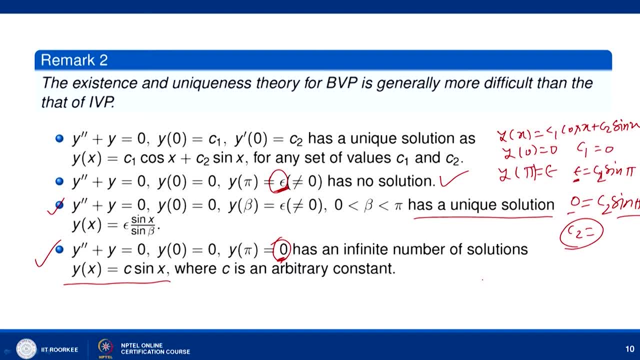 epsilon sin x upon sin beta. that also you can get it from This. so you can say that y0 equal to 0 means c1 equal to 0. so it means that now we have yx equal to c2 sin of x and y beta is equal to epsilon is given, so epsilon is equal to c2 sin of beta. 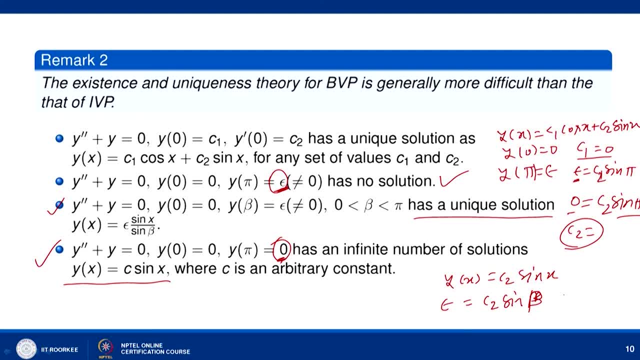 So c2 sin of beta you can get. so c2 is what epsilon upon sin of beta. So solution is given as yx equal to epsilon sin x upon sin beta and this is a unique solution. so it means that if you change your Solution, 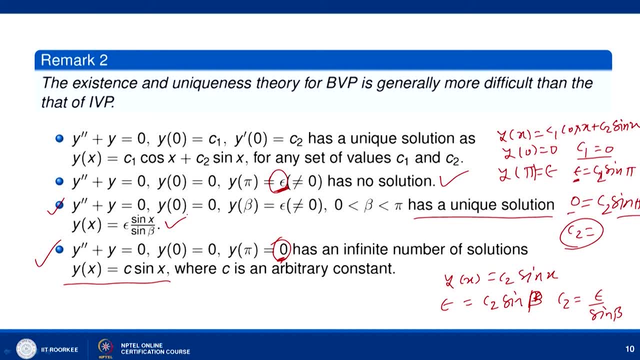 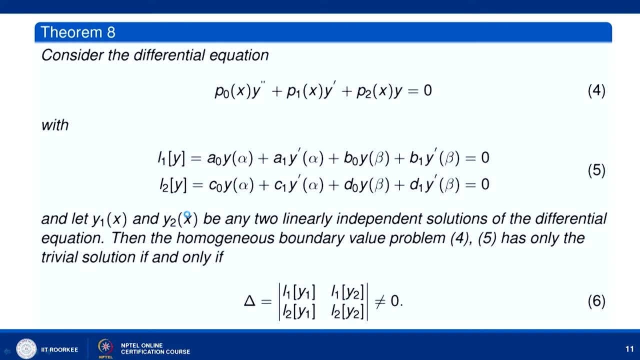 Solution, Boundary condition a bit and you have all the cases that no solution, unique solution and infinite many solutions. So it means that here we have to look at our existence and uniqueness theory in a very careful manner. So now let us start with the simplest possible cases. The simplest possible is the homogeneous. 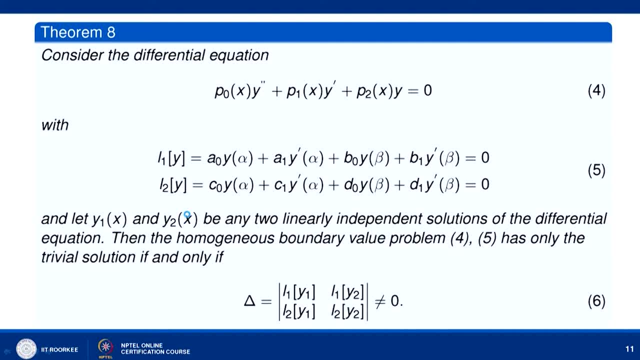 equation with homogeneous boundary condition, and we know that a homogeneous boundary value problem has a trivial solution. So we say that consider the differential equation this: p0 xy, double dash plus p1 xy, dash plus p2 xy, equal to 0, with the boundary condition l1 y, which is defined like this. So l1 y is: 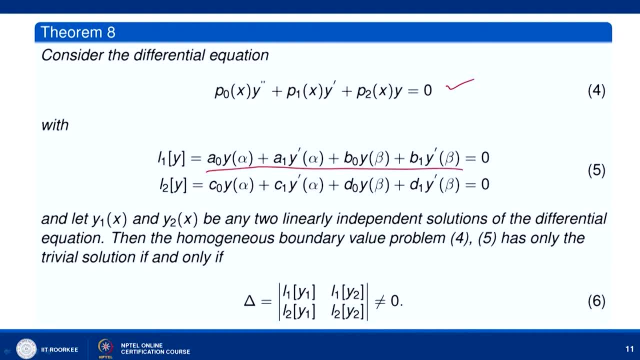 defined as a0 y alpha plus a1 y dash alpha, plus b0 y beta plus b1 y dash beta, equal to 0.. So we can summarize this to write: l1 y equal to 0, and similarly this as l2 y equal to 0. 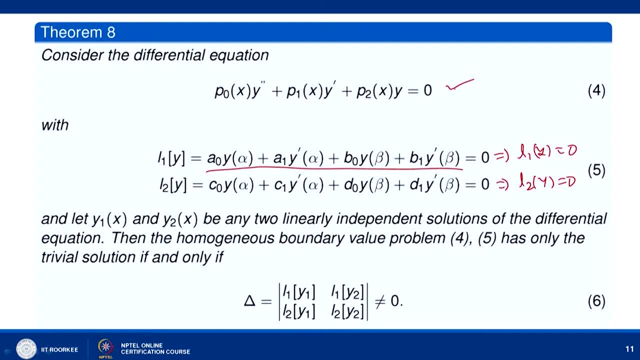 So we have a homogeneous solution. So we have a homogeneous solution. So we have a homogeneous solution. So we have a homogeneous differential equation and homogeneous boundary condition and we already know that 0 solution satisfy this. but we are interested in finding the non-trivial solution. 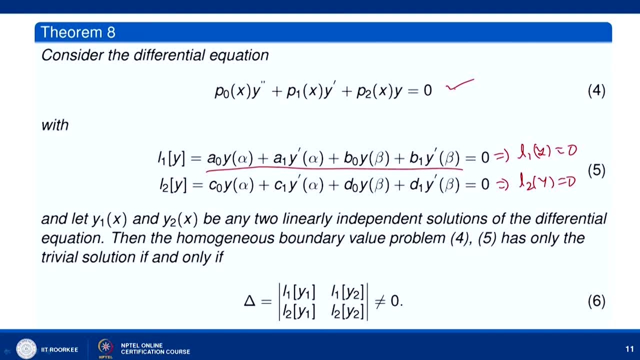 In trivial solution already exist. that is 0 solution. Now how to find out non-trivial solution? So we try to first find out the condition under which we have a non-trivial solution for this homogeneous boundary value problem. So for that let y1 and y2 be any. 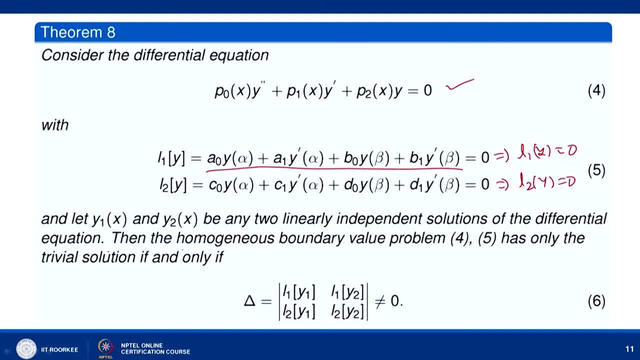 two linearly independent solution of the differential equation. So we have a non-trivial solution. So the nth equivalent of 1 n is 0 about 1, If only if this term is, this quantity is different from 0. If this quantity is equal to 0, then 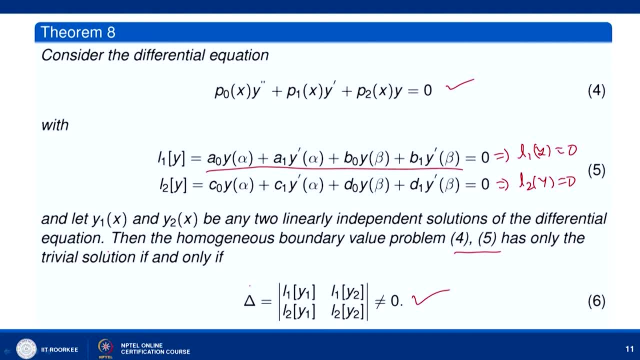 we may have more than one solution, but in case when this quantity delta is non-zero, then we have only, and only trivial solution. So let us prove this. So proof is quite simple. Let us start the analysis. Okay, so we have a actually Helix 3 很. 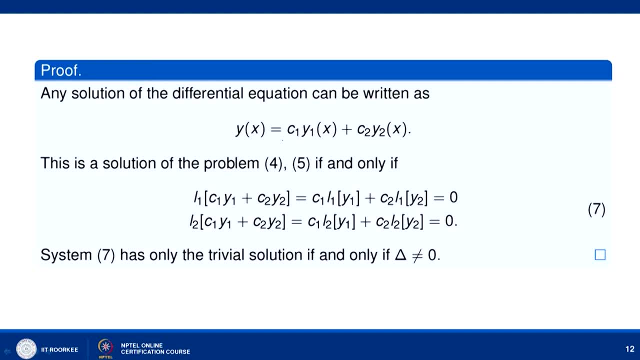 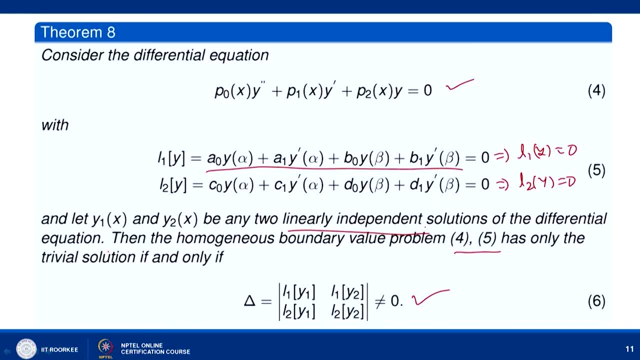 you simply say that your general solution is written as yx equal to c1y1x plus c2y2x, because it is already given that y1 and y2 are two linearly independent solutions. So general solution, you can easily find out. So general solution is given then. Now we can. 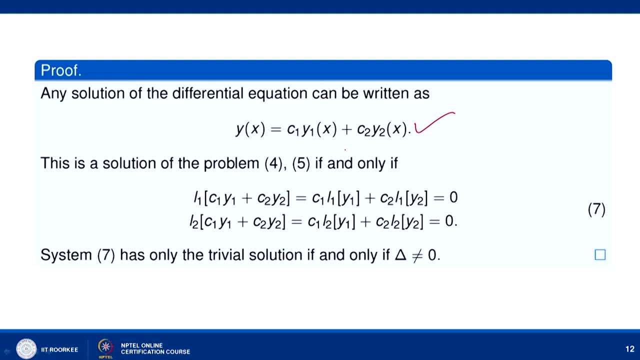 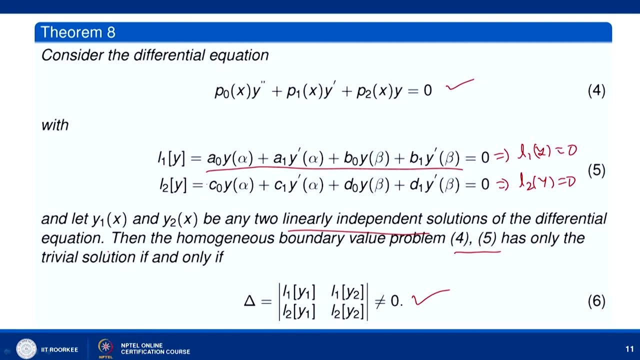 find out c1- c2 using the boundary condition. So if you use boundary condition, then L1 of c1y1 plus c2y2 is c1L1y1 plus c2L1y2 equal to 0.. Please look at here your boundary condition, which is defined as L1y and L2y. This is a 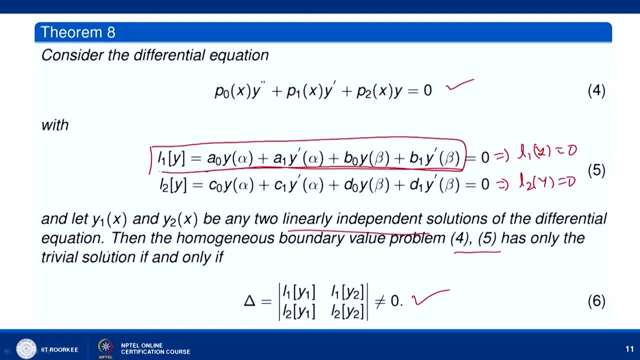 linear form, I will say It means that this is a linear in terms of your y alpha, y dash alpha, y beta and y dash beta. So it means that I can easily check, In fact I request you to check, that L1y is a L1y and L2y are linear, are linear in terms of the boundary. 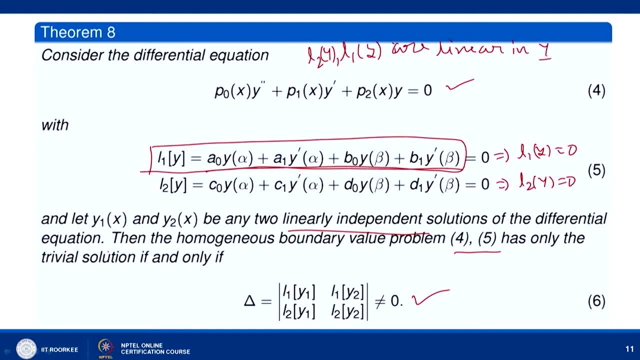 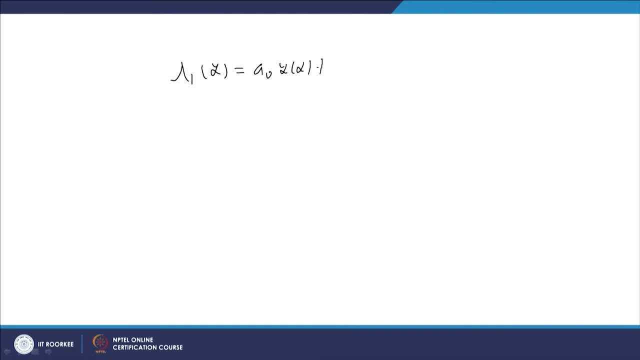 condition in argument. that is y here. How you can check. You look at here. So let me write it: 1. L1y equal to a0y alpha plus a1y dash alpha plus b0y beta plus b1y dash beta, and we want to check whether it is linear. 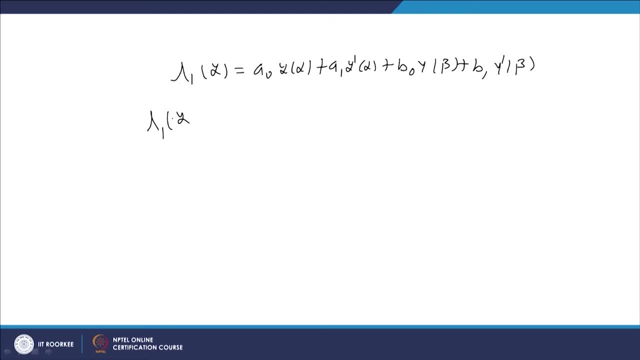 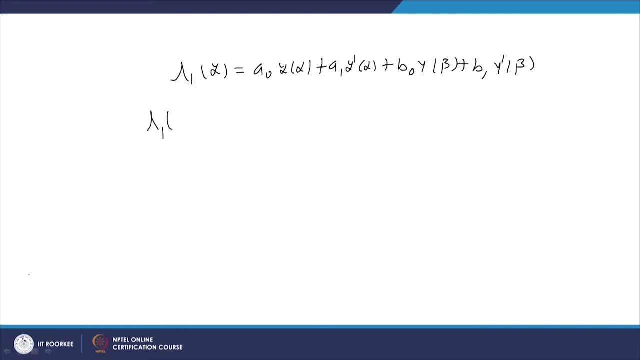 alpha. We have already taken alpha, We have already taken alpha, So let us use some other. So let us say, you say R1 and R2.. So let us say R1y1 plus R2y2 and we want to check whether. 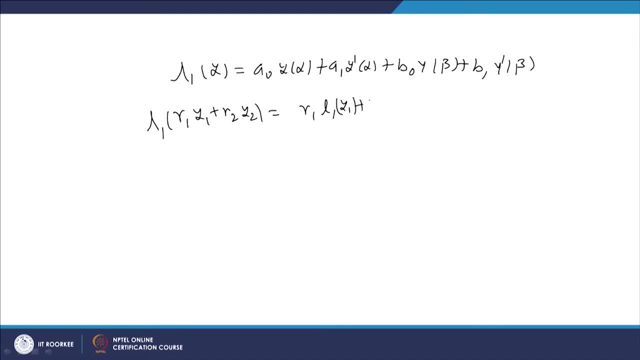 it is R1 L1 of y1 plus R2 L1 of y2.. If it is, then we say that L1 is a linear in terms of y and that you can easily check that it is actually satisfying this. Let me write. 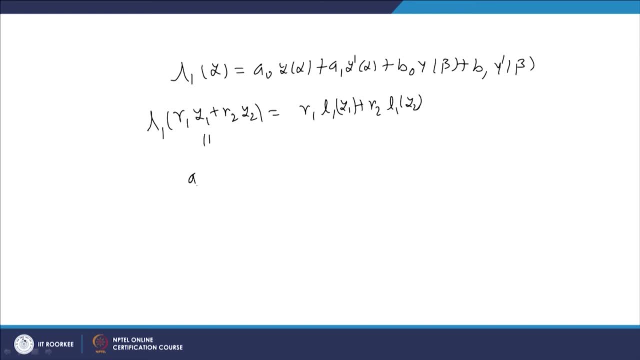 it here. So this is what. Now. this I am writing as a0y alpha is R1y1 plus R2y2 defined at alpha, plus a1. R1y1 plus R2y2- dash alpha, plus b0. R1y1 plus R2y2 defined at beta, plus b1. R1y1 plus R2y2 dash alpha. 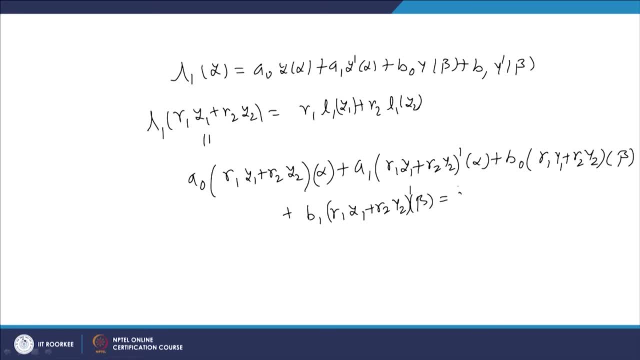 Now this: if you simplify, it is what Here R1y1 plus R2y2 given at alpha is what R1y1 alpha plus R2y2 alpha. So we can simplify and we can write it R1 and here we have a1. 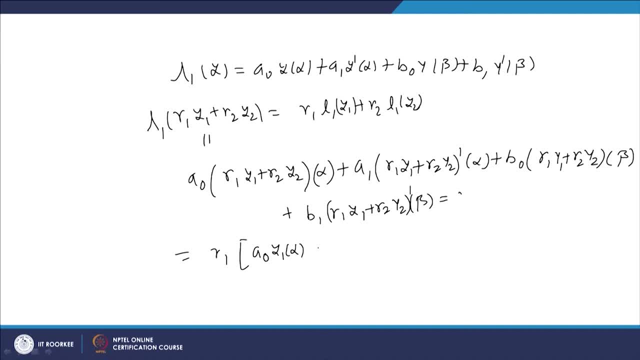 a0y1 alpha that you can easily check. So this we are taking and here we are taking. So here we have b1y1 dash alpha plus- look at this term. Here we have b0y1 beta plus. here We have b1y1 dash beta plus. look at R2.. So here, R2- look at the last term. So here, if you look, 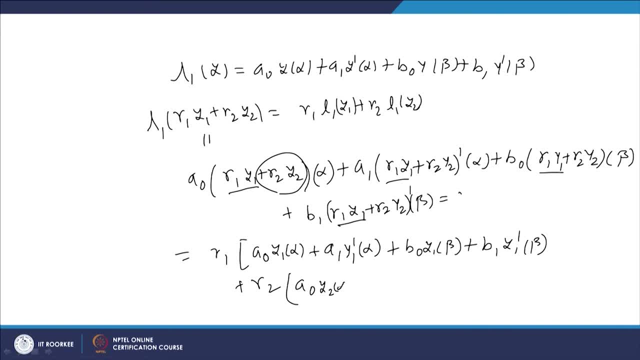 at this. then we have a0y2 alpha plus- look at this term, So it is y2- dash- alpha plus. look at this term. So here we have b0y1 into a1 plus this term, that is b0y2- beta plus this term, that is b1y2. 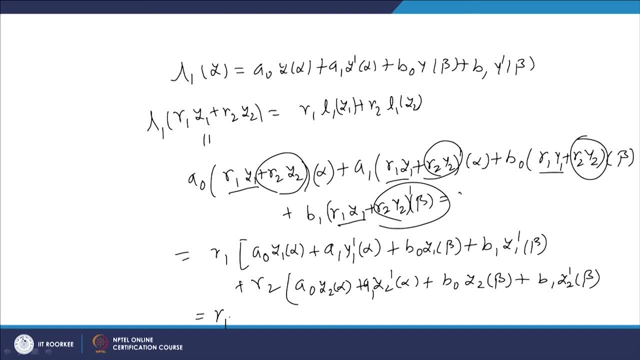 dash beta. So this is what R1 and if you look at this, is what L1 in terms of y1 plus R2.. Now look at this: This is what L1y2.. So we have proved, or we have shown, that L1,. 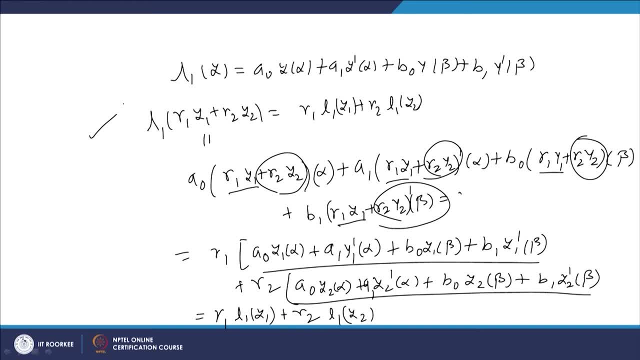 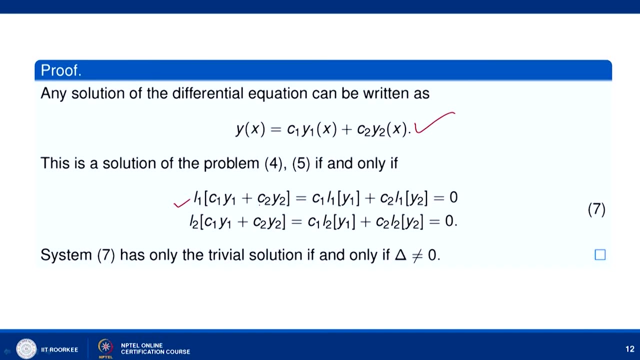 R1, y1 plus R2.. So it means that L1,. similarly, we can prove that L2 also is linear in terms of y, So we are going to utilize this. So here we simply say that L1 of c1y1 plus c2y2.. Now, using linear 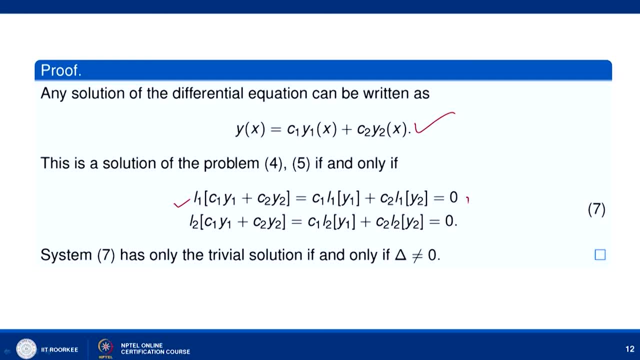 activities. what c1 L1 y1 plus c2 L1 y2, equal to 0, and L2 c1 y1 plus c2 y2 is equal to c1 L2 y1 plus c2 L2 y2, equal to 0.. 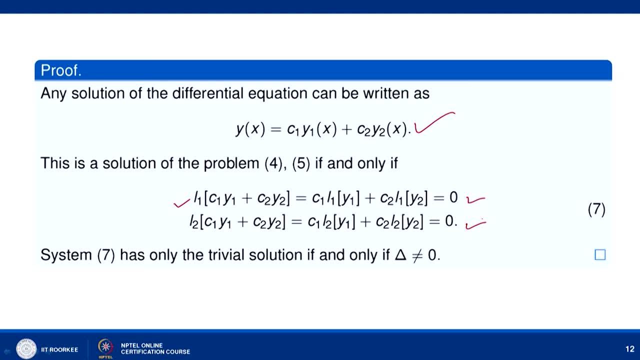 Now to find out a non-trivial solution. we must have that we should have a non-trivial value of c1 and c2.. Non-trivial values of c1, c2 means non-zero values of c1 and c2.. So here we have this and L1, so we simply say that we will get a non-zero value, provided. 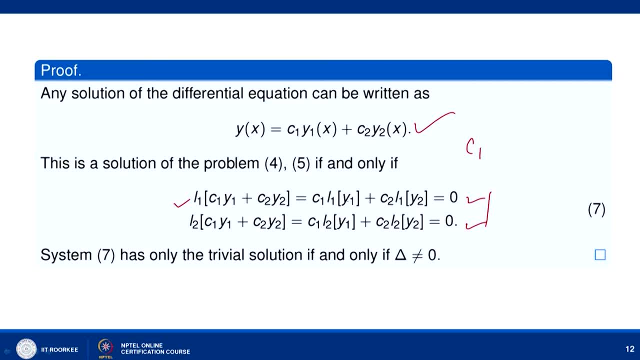 this c1. And let me write this equation right. So this is what Ax equal to B, kind of thing. So here we have c1, c2 and like this, And here we have what L1, y1, L1, y2, L2, y1, L2, y2, and here. 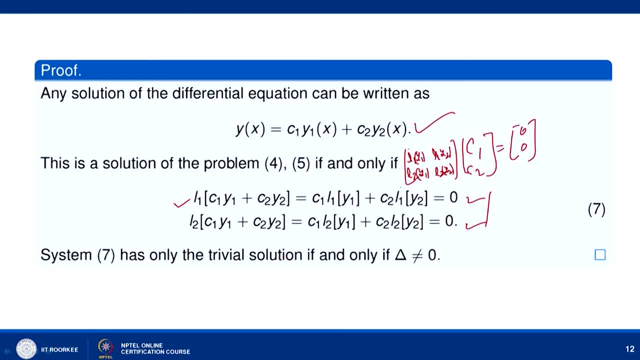 we have 0, 0. So we have Ax equal to 0 kind of thing. So here this will have only a trivial, trivial solution, provided that determinant of this coefficient is basically nonzero. So we say that this system has a only trivial solution, provided that determinant is nonzero. 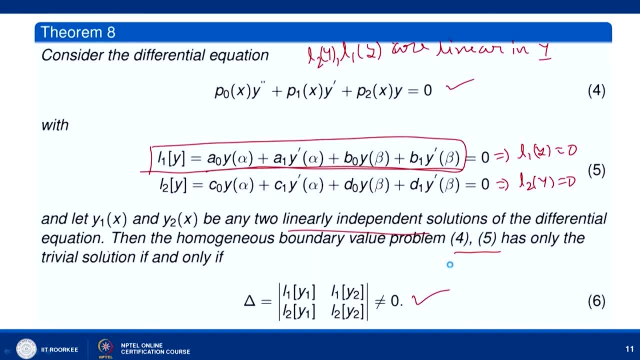 right. So that is the content of this theorem- that this homogeneous boundary value problem will have a trivial solution if, and only if, this quantity delta is nonzero, determinant of this value is nonzero. So if it is 0, then we may have more than one solution, In fact. 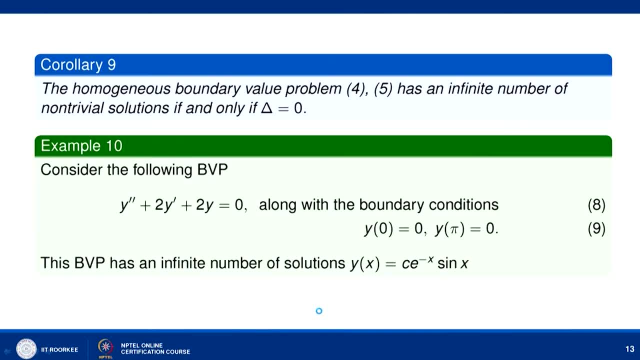 we may have infinite many solutions. So that is the content of this corollary: that the homogeneous boundary value problem has infinite number of non-trivial solution if, and only if, delta is equal to 0.. So we have just taken the half way. you have to prove the remaining part. 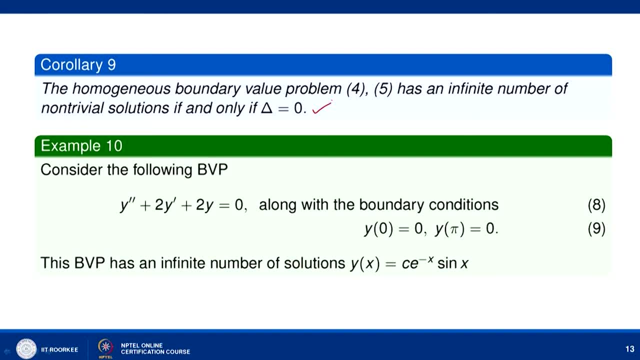 So we have just taken the half way. you have to prove the remaining part. So we say that if delta, that quantity is 0, then we have infinite solution. If delta is nonzero, then we have only a trivial solution. but it will always have a solution. 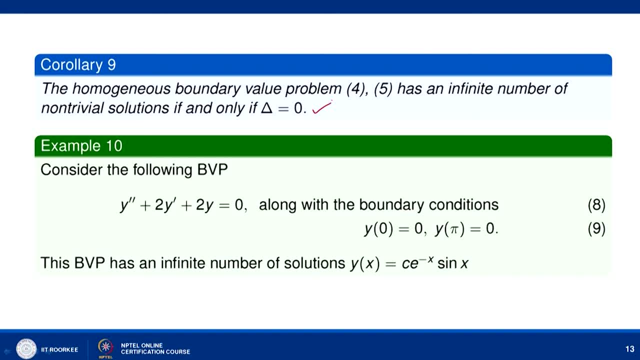 So let us consider one example, that is, y double dash plus 2y. dash plus 2y equal to 0. Boundary condition is given as y0 equal to 0 and y pi equal to 0, and to find out the solution here, we have to find out the solution here. So we have to find out the solution here. 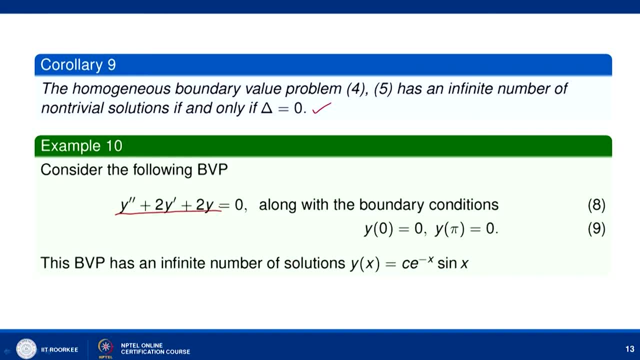 we simply first find out the general solution of this. For finding the general solution of this we can use, we can find out the solution by given method. So here you can simply say that here solution is given as e to the power minus x sin of x, you can call it y1 and y2 as e to the power. 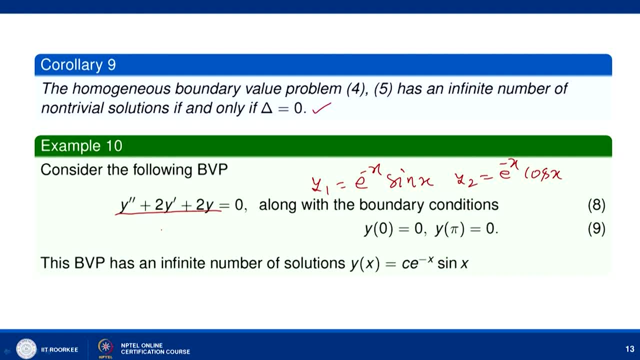 minus x cos of x. That you can simply check that. it is what you can write it. your auxiliary equation is x sin of x. So that is what you can write it. Your auxiliary equation is x sin of x. m square plus 2m plus 2 e to the power mx equal to 0 and it is m plus 1 whole square. 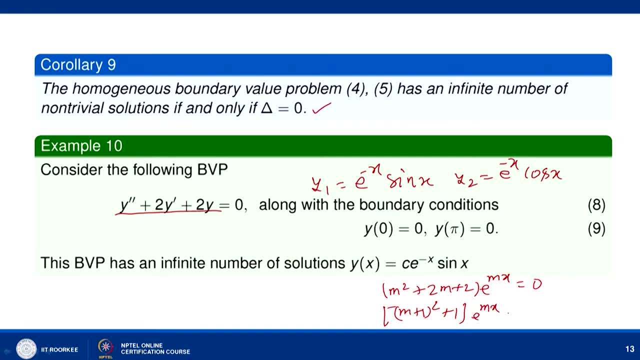 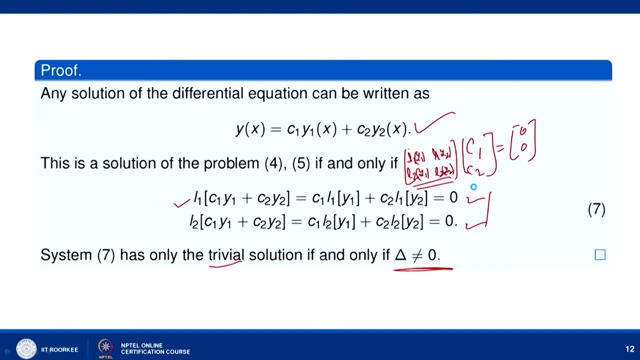 plus 1 e to the power mx equal to 0. When you put y as e to the power mx as a solution here, then you will get this as a solution. So this quantity has to be 0 and using the boundary condition you can fix it. But if you look at here- I just want to go back again- because here, if you, 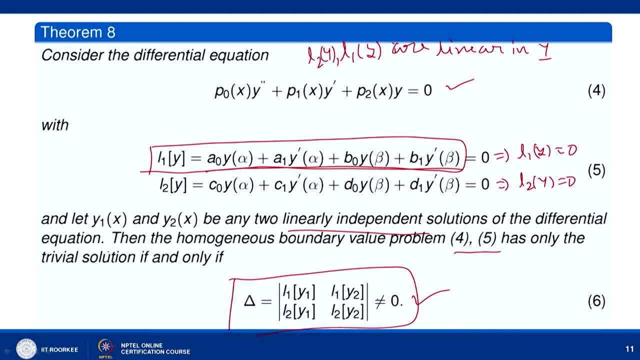 look at this is depending on the boundary condition. basically It is not depending on, say, solutions. Here you take y1 and y2: are any two linearly independent solution? but this delta is depending on the boundary condition rather than specific, initial, specific solution of 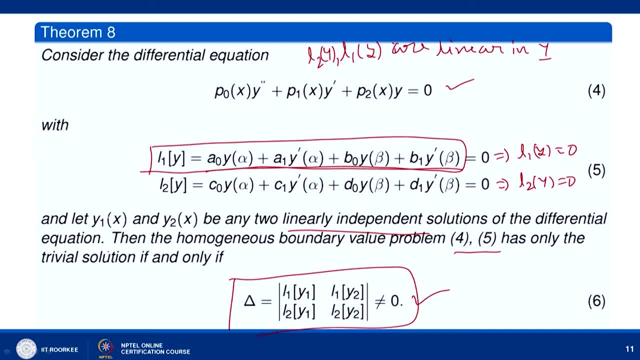 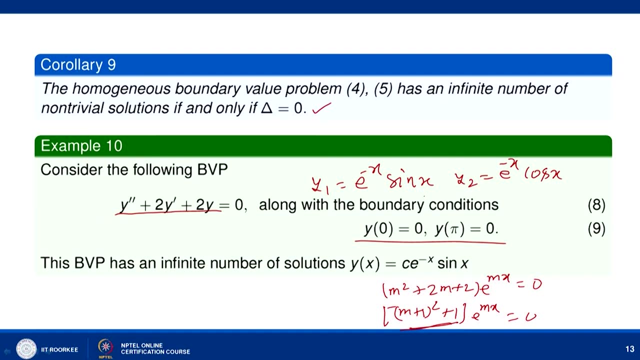 this boundary value problem. So it is very much centric about the boundary condition rather than your solutions. So here you can take any two linearly independent solution and you can easily check this. So let me take solutions as e to the power mx sin x and e to the power mx cos of x and that you can easily check. So general solution. 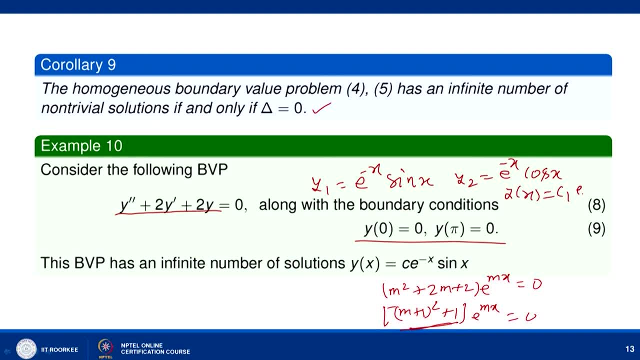 you can find out y of x equal to c1, e to the power mx sin of x, plus c2 e to the power mx cos of x. So we have already condition l1y equal to 0.. So you can look at the delta here. Delta is what? 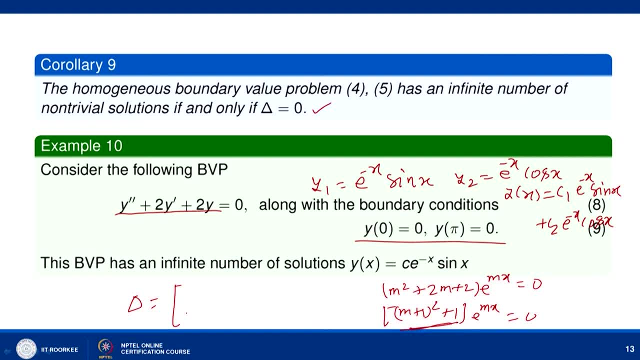 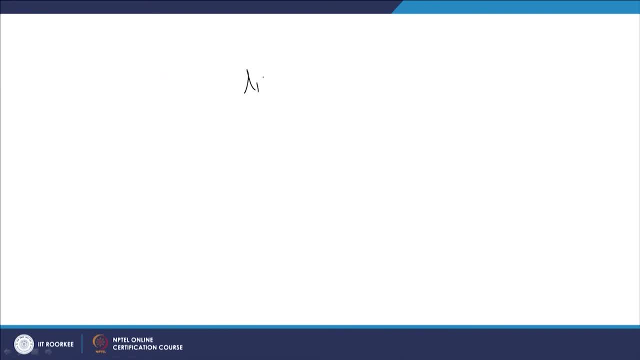 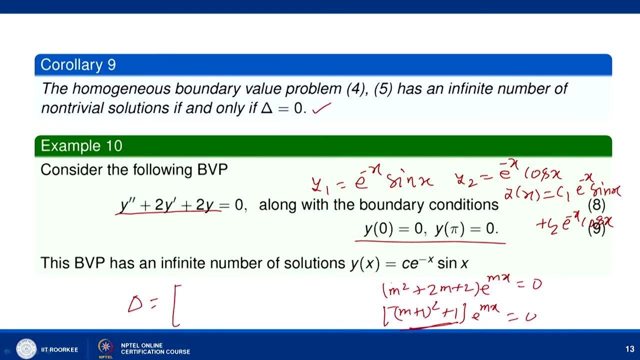 l1,, so let me write it. What is l1 here? l1y is y, Let me write it here. So here l1y is basically y at 0, right and l2y is y of pi. 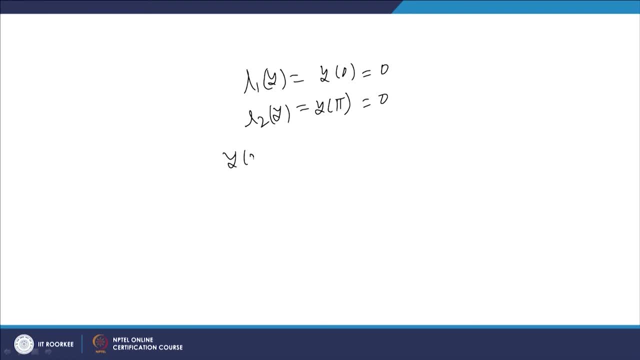 So l1y1 is basically what e to the power mx cos of x plus c2 e to the power mx sin of x and yx is already given: c1 e to the power mx cos of x plus c2 e to the power mx sin of x. So we can easily check. l1 of y1 is basically: 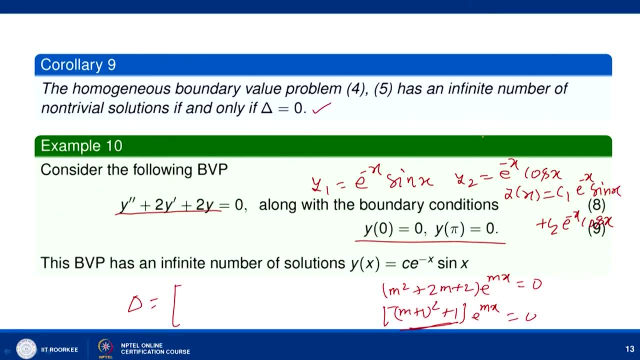 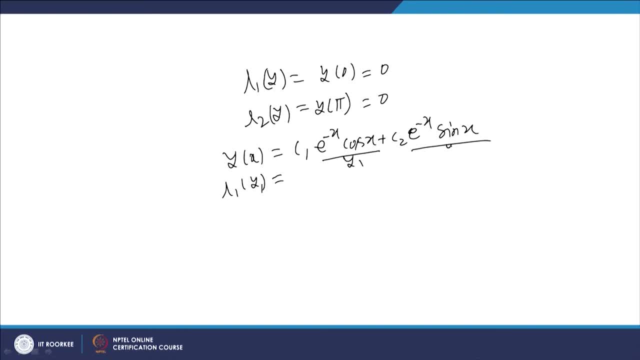 what? y1 is this? y2 is this. Let me see whether what I have defined okay, so you can easily check what is l1, y1.. So let me write it: y1 is this, y2 is this. So l1, y1 is basically what? e to the. 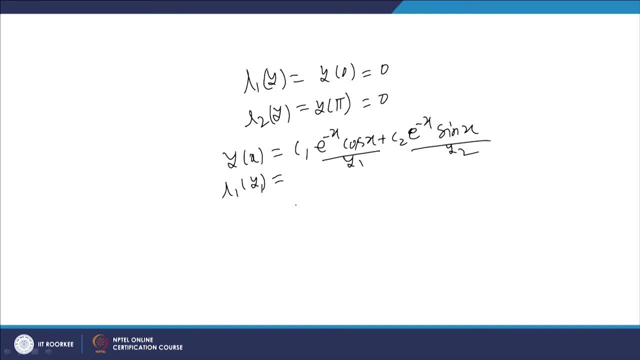 minus x cos x. define at 0. So that is going to be what It is going to be: 1 only Is it okay. Now, L1 of y2 is what L1 of y2 is going to. what Define this at 0. So this is going to be 0. Then. 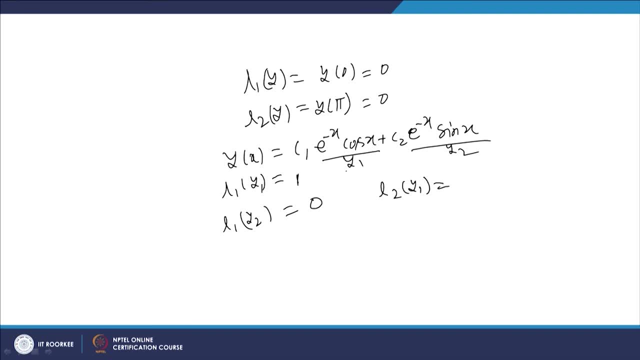 L2 y1,. L2- y1 means this define at pi. So it is e to the power minus pi. cos of pi is minus 1, so it is minus L2 of y2 is going to be again 0.. So now look at the determinant. Determinant is L1. 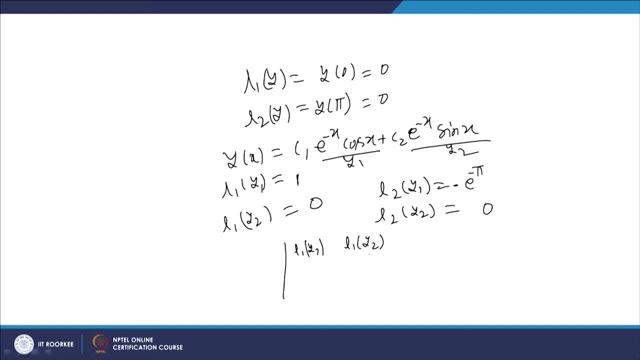 y1, L1 y2, L2 y1, L2 y2.. That determinant we are. this is your delta. So this L1 y1 is basically 1, L1 y2 is 0, and this is what e to the power minus minus of e to the power pi, and this is 0. 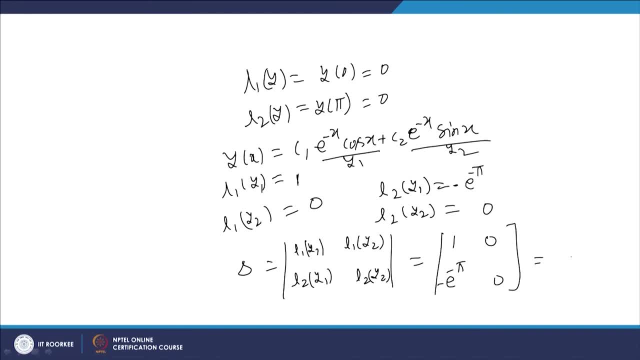 And you can see that it is having what? E to the power pi, E to the power pi, E to the power pi. It is 0 basically. So it means that this delta is coming out to be 0.. So it means that our theory. 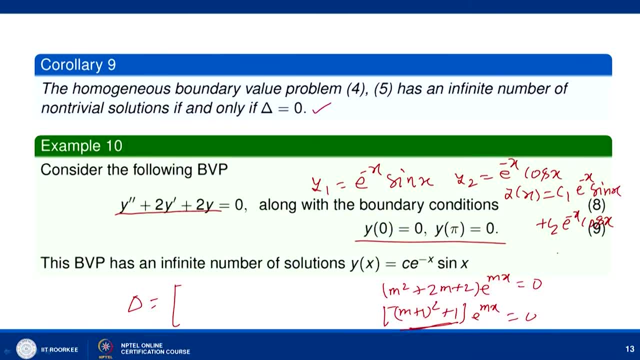 says that it has infinite many number of solution and you can easily check that your infinite many solution is given by yx equal to c into e, to the power minus x sin of x. How can you check that? So this theorem simply says that it has infinite many number of solution? How to find out That? 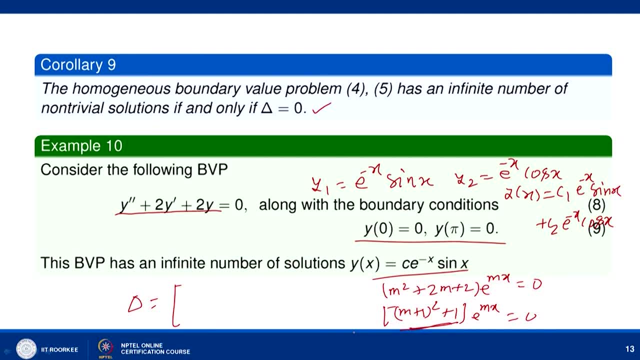 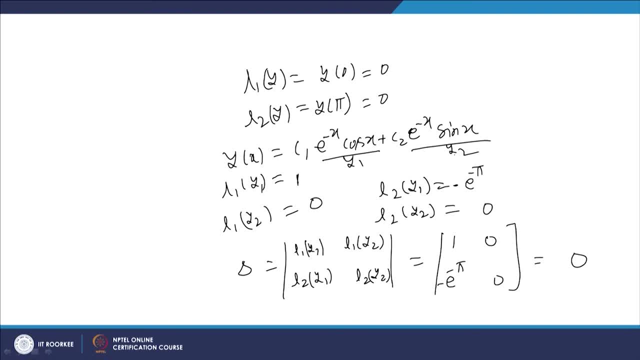 is up to you Means you have a general solution and you have boundary condition. you can easily find out the solution. Let me say that here your condition, your general solution, is this: Then y0 equal to 0 means here you simply say that: 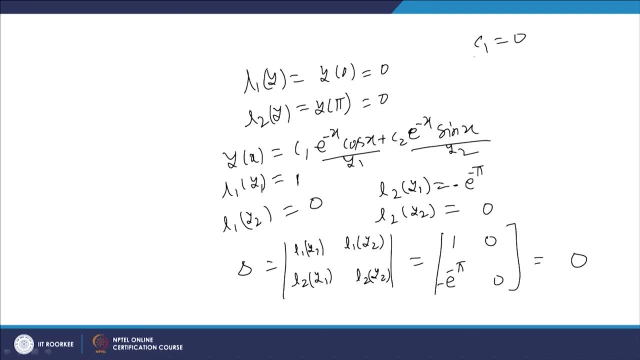 c1 has to be 0, using y0 equal to 0. Now ypi equal to 0, let us use this and how to see Then. this is what c1 is: 0 means only c2. is there So c2 e to the power minus pi here and sin of pi. 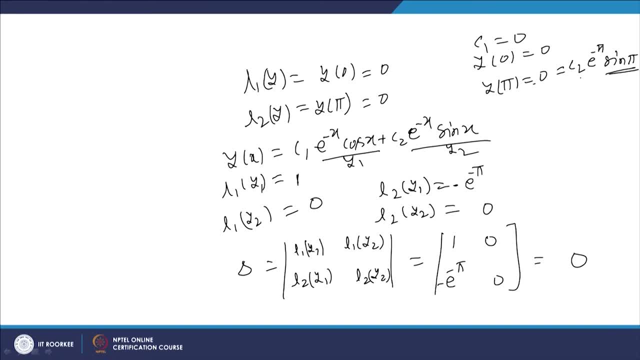 sin of pi is simply 0. So 0 equal to c2 into 0. So c2. you can take any value. So you can take any value. So let us say k belongs to R. So here we simply say that your solution is c, e to the power minus. 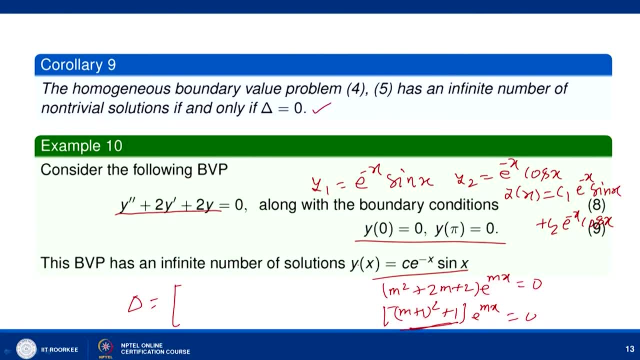 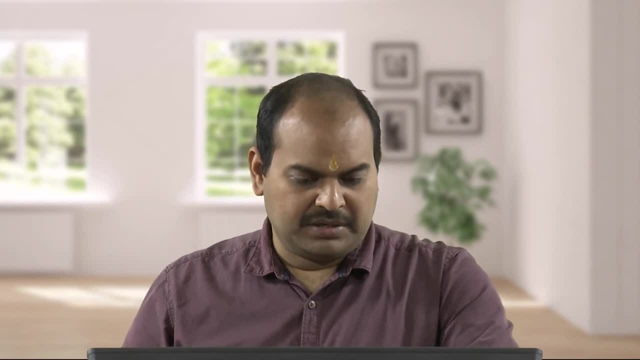 x, sin of x and c is coming from R. So we can say that here we have infinite many solution. and given by this and this we have checked using delta- Here delta is coming out to be 0 and so we have infinite many solutions. So we have seen that in a homogeneous boundary value problem, when we have 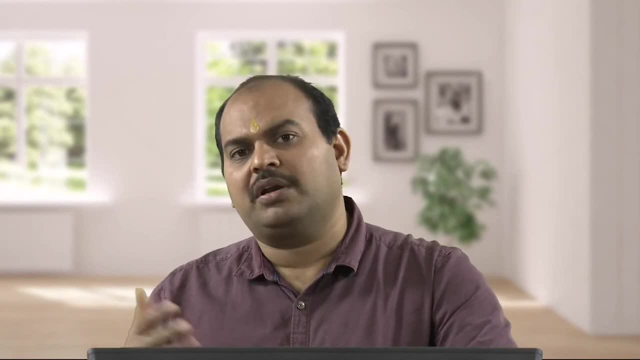 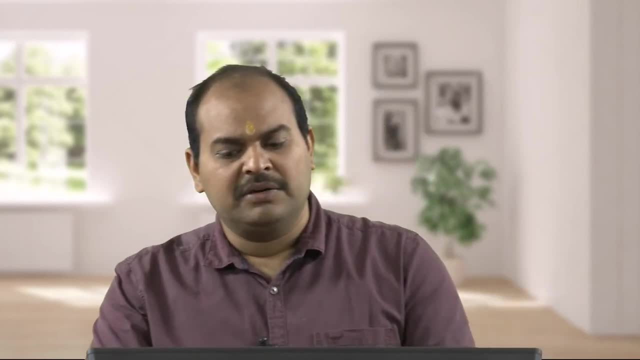 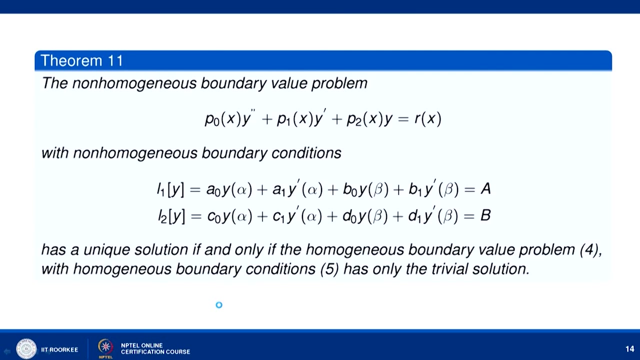 Now let us look at the non-homogeneous boundary value problem with non-homogeneous boundary conditions. So the non-homogeneous boundary value problem- p0xy double dash plus p1xy dash plus p2xy, equal to R of x and non-homogeneous boundary condition is given: l1y equal to a and l2y. 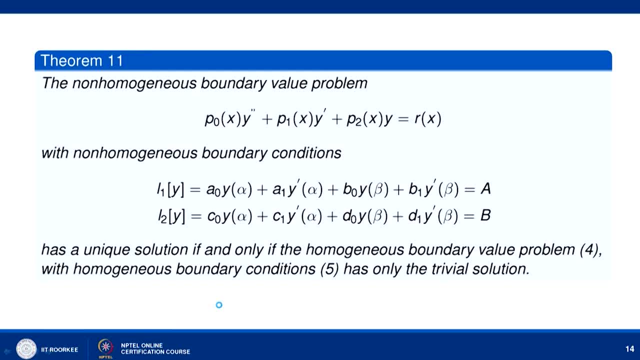 equal to b. This has a unique solution if, and only if, the homogeneous boundary value problem with homogeneous boundary condition has only the trivial solution. So that is why whatever we have discussed is going to be very useful in finding the solution: unique solution for a non-homogeneous boundary value problem. 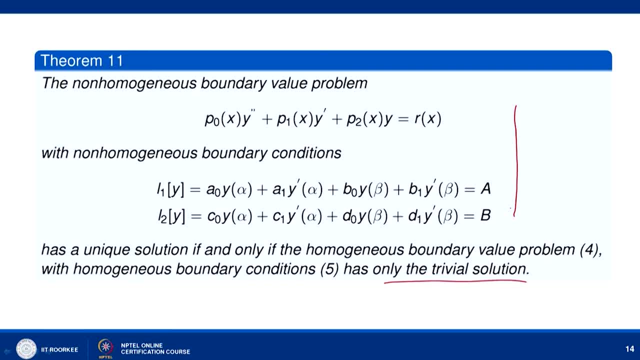 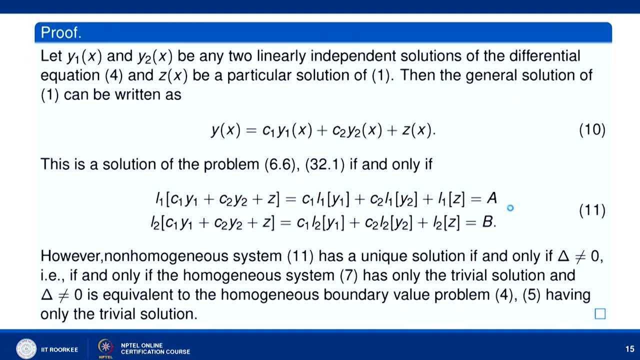 So if we have a homogeneous boundary value, problem has a trivial solution, then non-homogeneous boundary value problem will have a unique solution. So let us say how the proof goes. So let us look at y1 and y2 be any two linearly independent solution of the 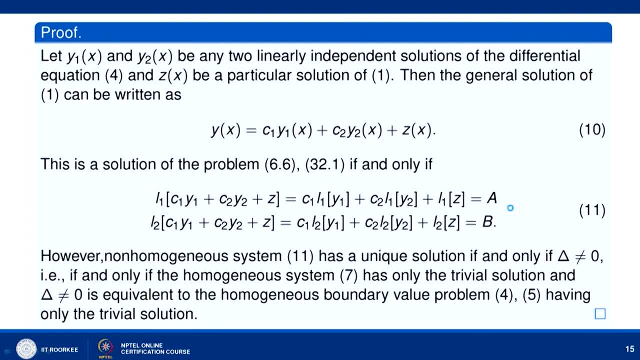 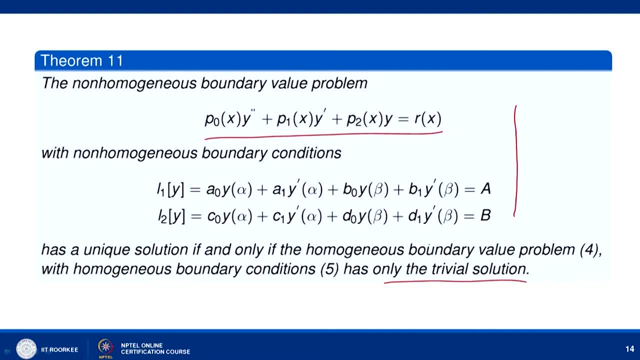 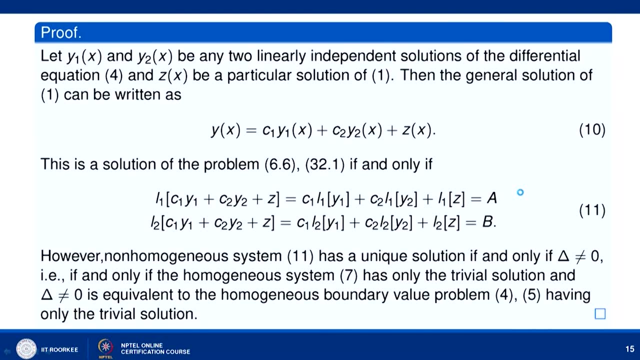 differential equation 4 means your homogeneous part and zx will be a particular solution of non-homogeneous equation. that is this: So zx is a particular solution of this non-homogeneous boundary value problem. this and it will satisfy this. So it means that then the 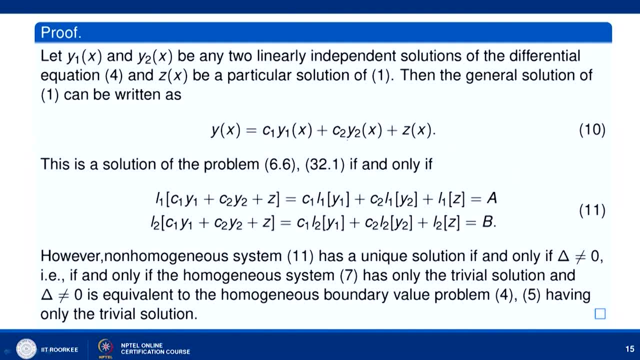 general solution of one can be written as: yx equal to c1, y1x plus c2, y2x plus z of x. So it means that this is a general solution of this, along with boundary condition. Now, since it satisfy the boundary condition, so we write: l1 of c1, y1 plus c2, y2 plus z equal to a. 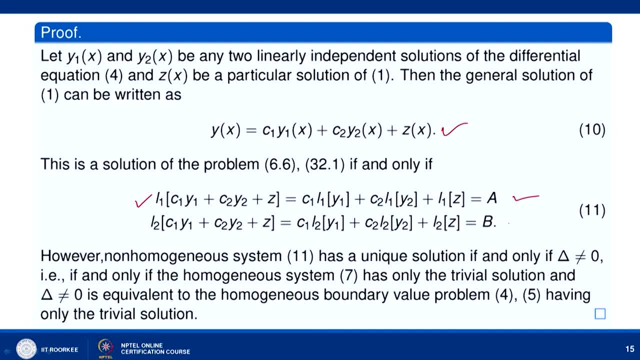 and l2, of c1, y1 plus c2, y2 plus z, equal to b. because, if okay, so it satisfy this condition, because y is a general solution of the non-homogeneous boundary value problem. So, if you simplify this, you simply say that since l1 z is equal to a and l2 z equal to b, 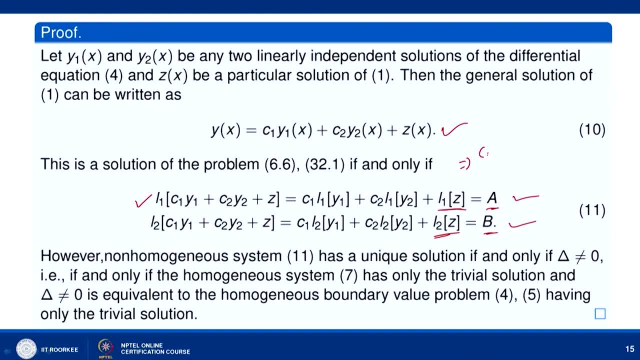 So this 11 equation, equation number 11, is due to this: c1, l1 y1 plus c2, l2 y2 is equal to 0 and c1, l2 y1. sorry, this is l1 plus c2, l2 y2 equal. 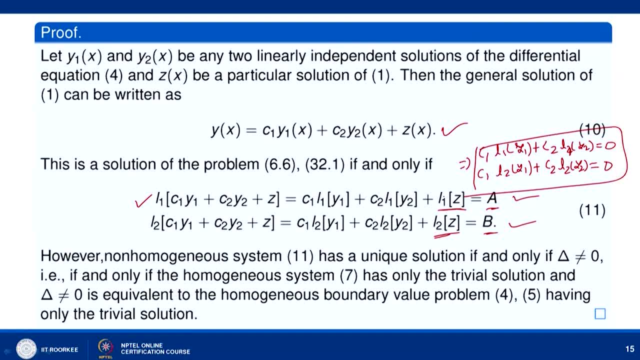 to 0 and, if you will remember, this is precisely the term we say that this equal to 0 means. this implies that this equations with all the non-ценzural factors, where we actually removenothing is homogeneous part, has a unique triple solution, provided that this delta, which is given as 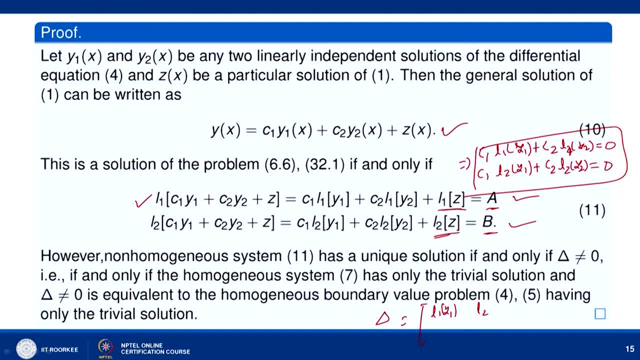 L1y1, L1y2,, L2y1, L2y2,. this determinant is non-zero. So if this determinant is non-zero, then you will have C1 equal to C2, we have a triple solution for homogeneous part. 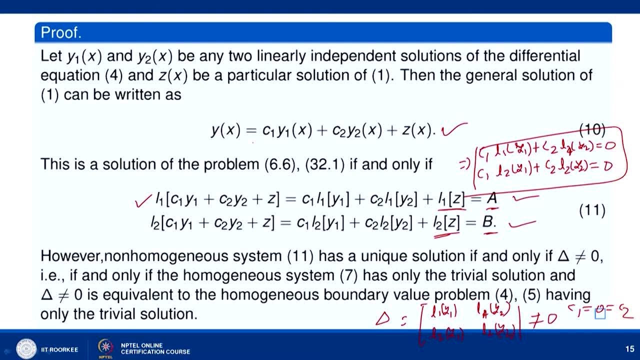 When you put a triple solution for homogeneous part, then this will simply say that this will cancel and we have yx equal to zx as the only solution. So we say that non-homogeneous system 11 has a unique solution if, and only if, delta is non-zero. because if delta is non-zero, 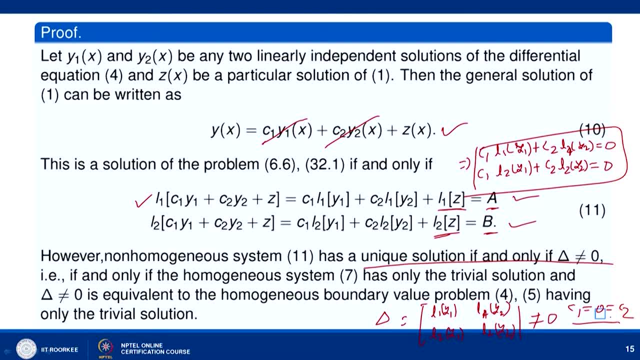 then we have C1 equal to C2 equal to 0 and we have only solution given as yx equal to z of x. So we can say that this non-homogeneous system has a unique solution if, and only if, delta is non-zero. and we can say that if, and only if, if the homogeneous system has only the triple solution. 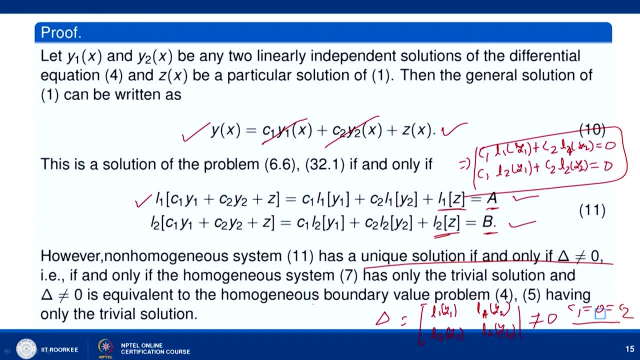 and delta is not equal to 0 is the equivalent to the homogeneous boundary value problem having only the triple solution. That is what we want to conclude from this equation. So from 11, you can conclude that triple solution for homogeneous boundary value problem is equivalent. 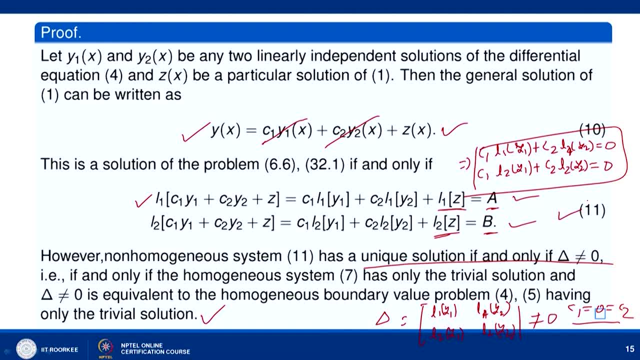 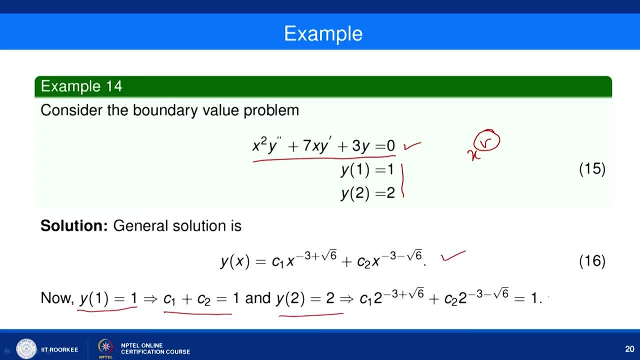 to say that we have a unique solution for non-homogeneous boundary value problem with non-homogeneous boundary condition. So let us take one example, One example based on this. So let us consider this example, Consider the boundary value problem. 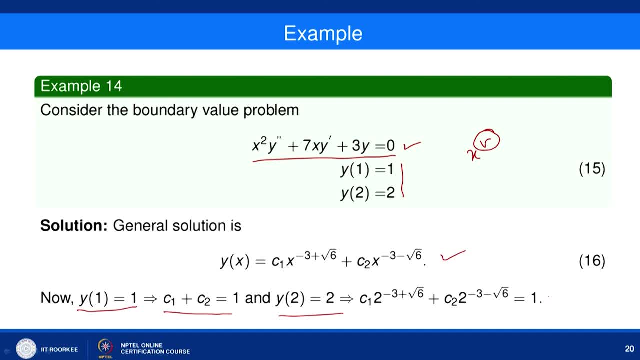 x square y, double dash plus 7xy dash plus 3y equal to 0, with the non-homogeneous boundary condition that is y1 equal to 1 and y2 equal to 2.. And we can simply say that, since it is a 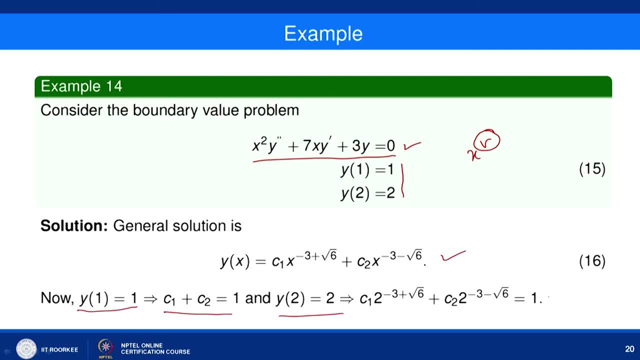 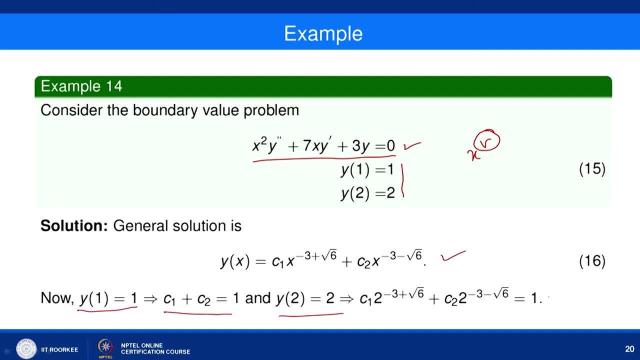 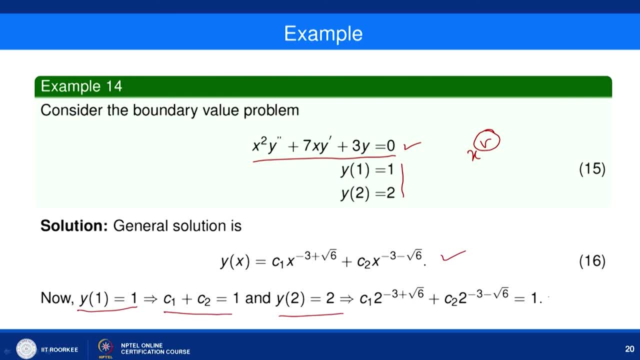 this. I am leaving it to you that how to find out a general solution of this. Now let us proceed further and we want to find out y1 equal to 1 and if you use the condition y1 equal to 1, then c1 plus c2 equal to 1 and y2 equal to 2 means c1, 2 to power minus. 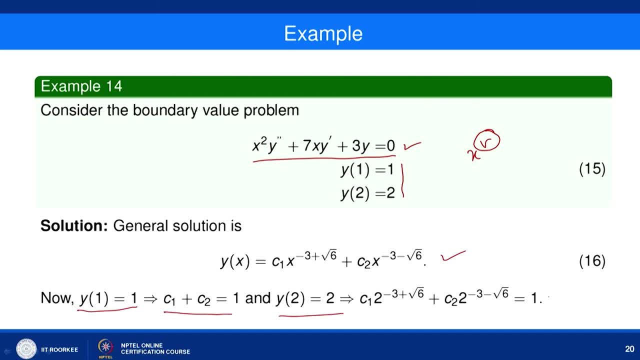 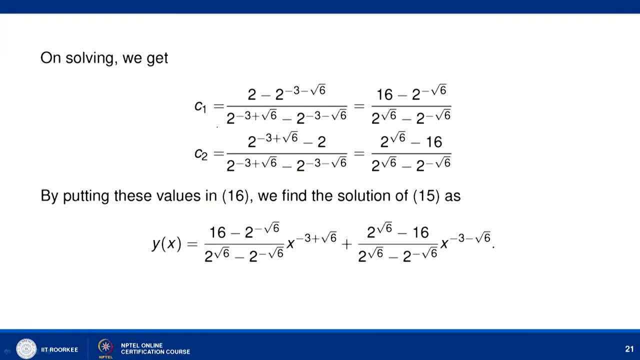 3 plus root, 6 plus c2, 2 to power minus 3 minus root of 6, equal to 1, and we want to find out the c1 and c2 for which it has a solution. So you just look at the value of c1,. 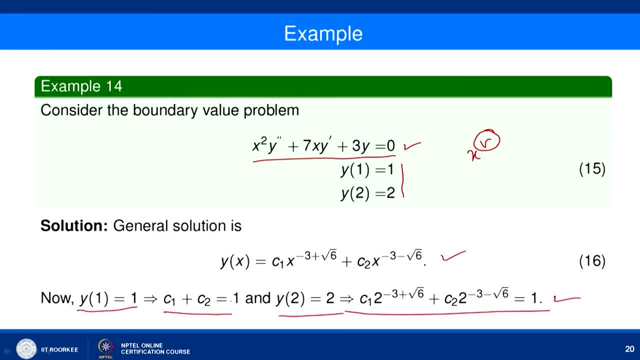 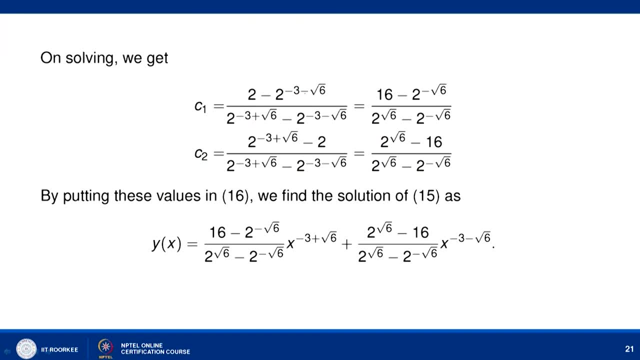 c1 is here. you can simply say c1 as 1 minus c2, put it back and you can simplify. So here you can get c1 as 2 minus 2 to power minus 3 minus root 6 divided by this quantity. 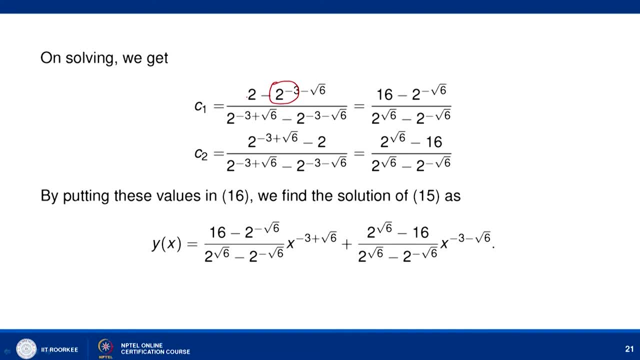 and if you simplify or you simply say that take this term out 2 to power minus 3 common, then you will get that c1 is 16 minus 2 minus root 6, divided by 2 power root, 6 minus 2 to power minus. 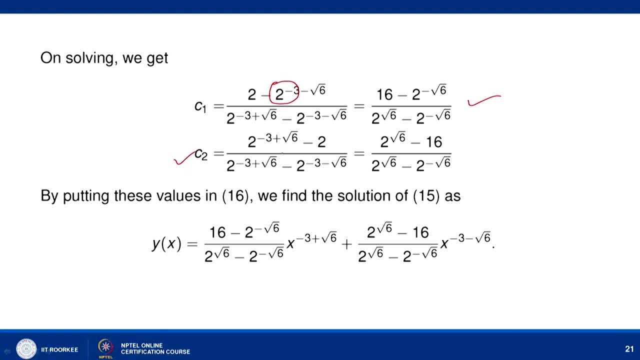 of root 6.. Similarly in c2 also, we take 2 to power minus 3 out and you will get c2 as 2 to power root 6 minus 16 upon 2 to power root 6 minus 2 to power minus of root 6, and once we have c1 and 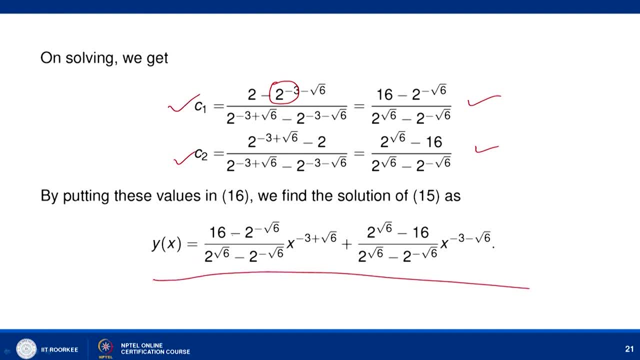 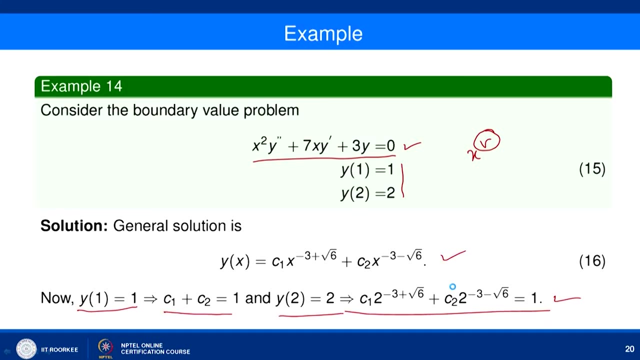 c2, you can write down the solution, general solution, as this: yx equal to this, and since now c1 and c2 are particular values, then we can call this as a solution of the initial value problem. So we can say that this is a unique solution of the boundary value problem here, and this we 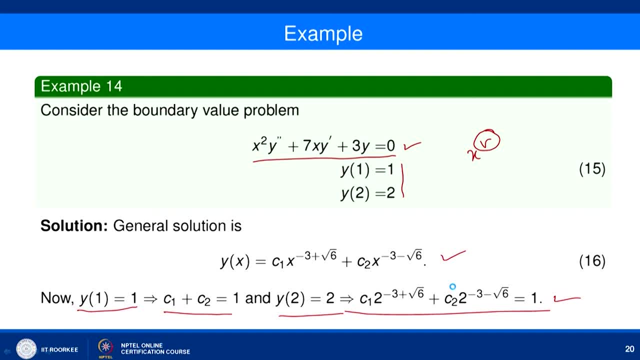 simply say that, since we are getting a unique solution because the homogeneous boundary value problem has a trivial solution. How we can check: You put y1 equal to 0 and y2 equal to 0, and when you put y1 equal to 0 and y2 equal to 0, then we have c1 plus c2 equal to 0 and c1- 2 to power minus.